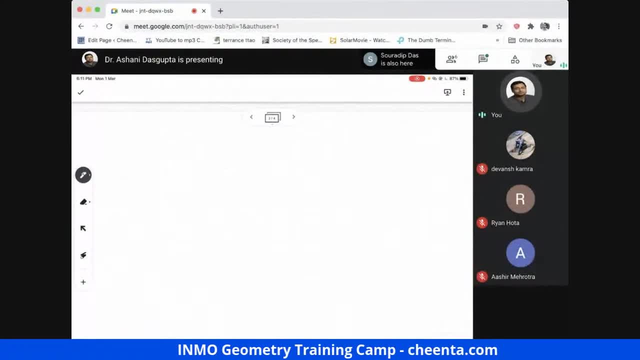 Okay, So basically to a different but related set of problems, and we will be starting with something called in circles And in circles and in red in red I. so this is a very important topic in geometry and problem solving in geometry. 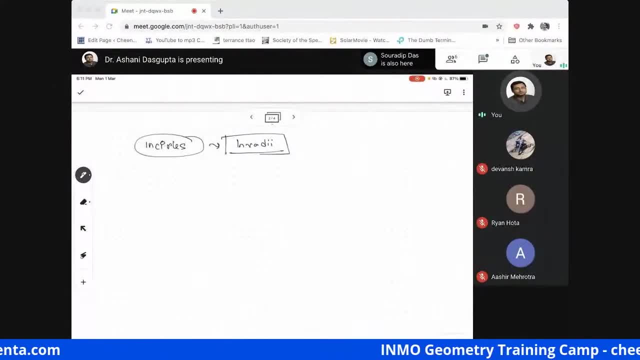 And to understand what we want, the theme that we want to talk about. we first talk about a problem like this. so it's a problem. one suppose we have a circle gamma. so gamma is a circle. let's draw it like this: and l is a line tangent to the circle gamma. so here is a line l which is tangent to the 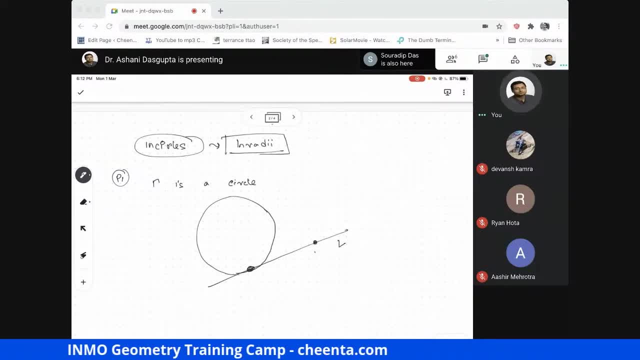 circle gamma and we have a point m on this line, l. so we want to find the locus of all points p with the following property: find the locus of p such that, such that there are two points, q and r, there are two points q and r on l, such that m is the midpoint of qr. 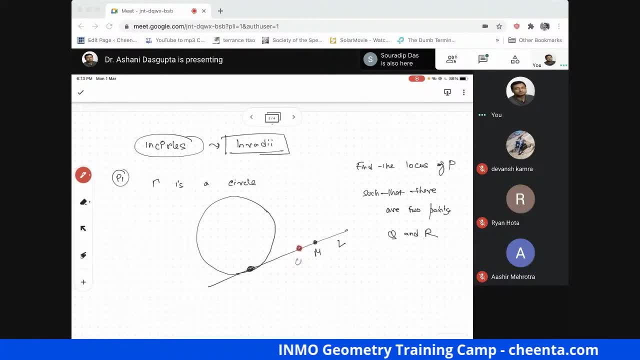 so maybe i can draw it in red, m is the midpoint of qr and gamma is the inscribed circle of triangle pq r. so gamma is the inscribed circle of triangle pqr and you can think of it. it's kind of weird because then you know that this particular picture wouldn't work. maybe you have to. 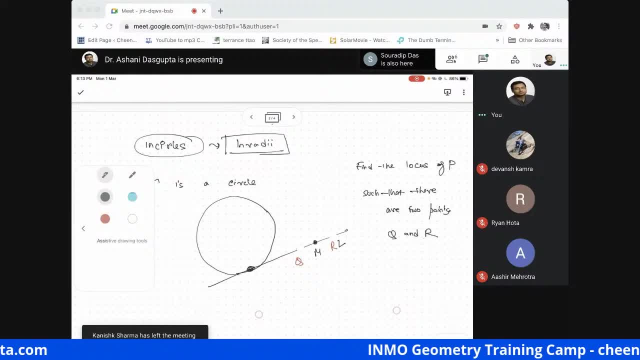 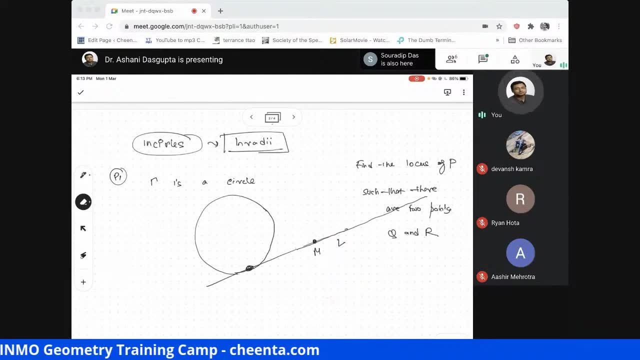 do it in a little bit different way. i will just extend it a little bit more. maybe i have to draw q here and i have to draw r here, such that pqr would be something like this. so i have drawn one such point p in this picture. i have drawn one such point p in this picture. 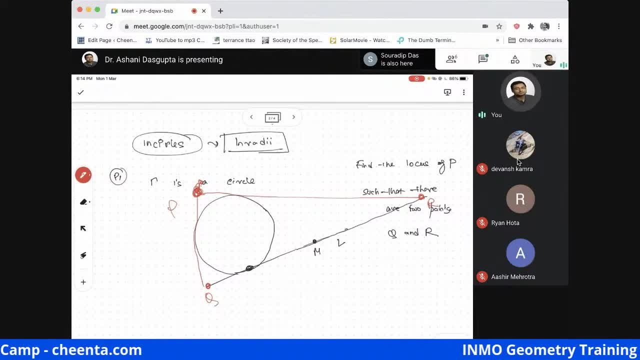 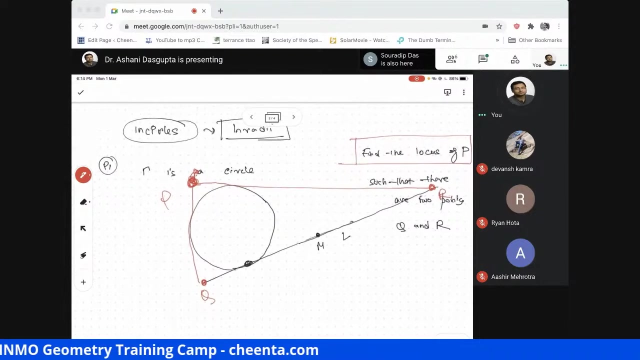 and i want to find out the locus of all such points p. find the locus of all such points p, not only one such point p. find the locus of one, just one point p. okay, so how would you go about it? do you understand this? you understand this problem, all of you. 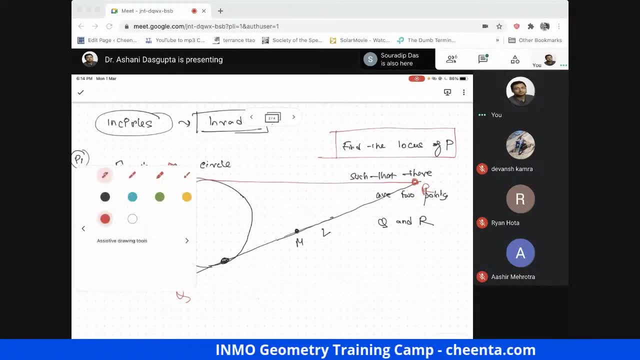 we start with the circle gamma, which we start with the circle gamma and we draw a tangent to the circle gamma. so this is in blue. draw a tangent to the circle gamma and draw and take and suppose the tangent line is l and fix a point m. fix a point m on the tangent. 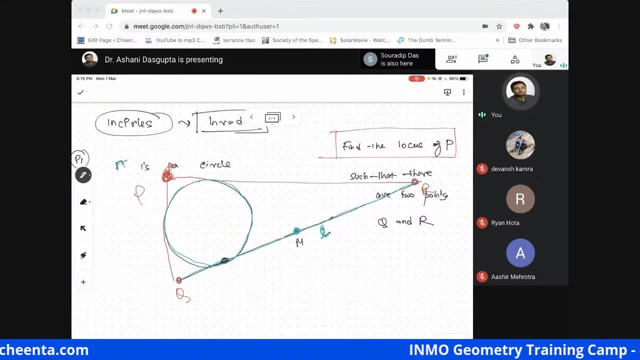 line. this is your given data. so your given data, your given data, is the circle gamma, is a tangent line. l and is the point m on the tangent line? the circle is a tangent line and we have a point m on the tangent line. we want to find out. point p: 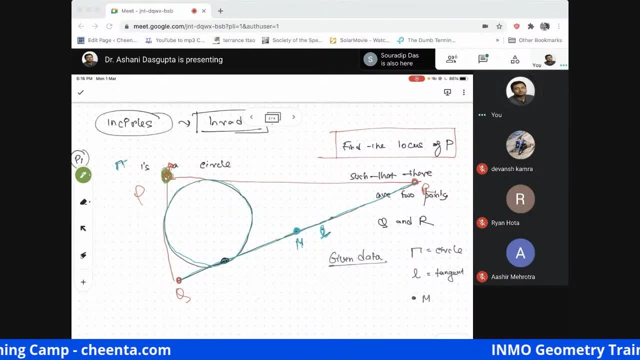 so let's draw that in blue, maybe find all such points p, find all points p, or rather locus of all such points, p, such that there are q and r. there are q and r, two points, so that m is the midpoint of qr, m is the midpoint of qr. 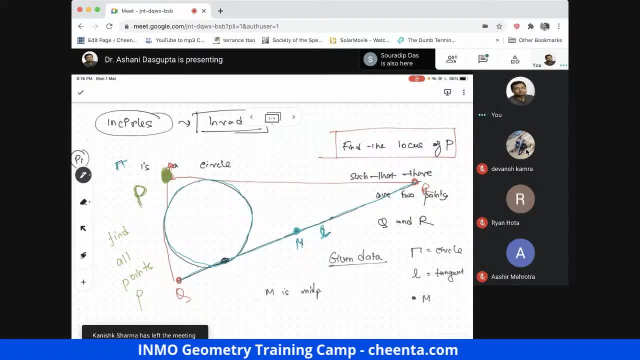 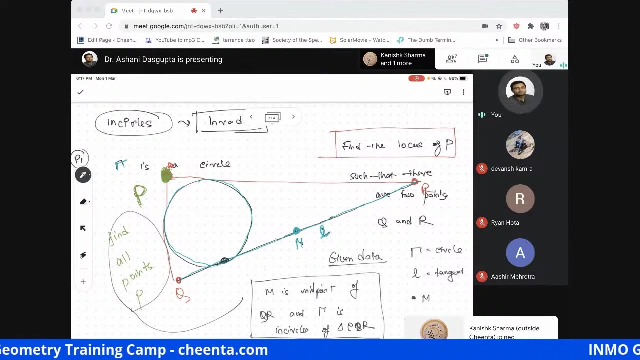 m is midpoint of qr and gamma is in circle of triangle pqr. so that's the property of P. find all such points, P with this particular property. so can you tell me how would you go about doing this problem? give it a try, all of you, sir. yes, sir, I think we can try coordinate geometry for this, because 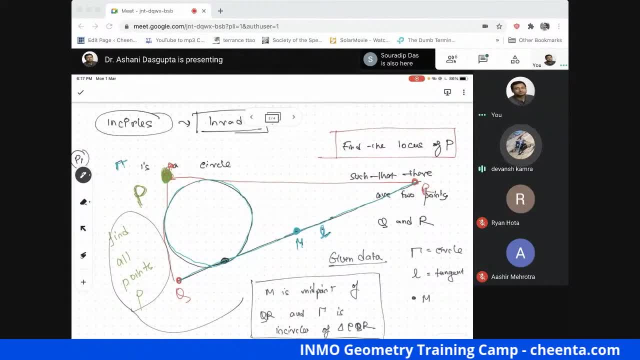 basically, P is the point of intersection of tangents from Q and R, and Q and R must be on the opposite ends of the circle gamma on the tangent line. okay, so maybe we can. so maybe we can try it using coordinate geometry, where the tangent line can be assumed as the x-axis, while the circle circle of the 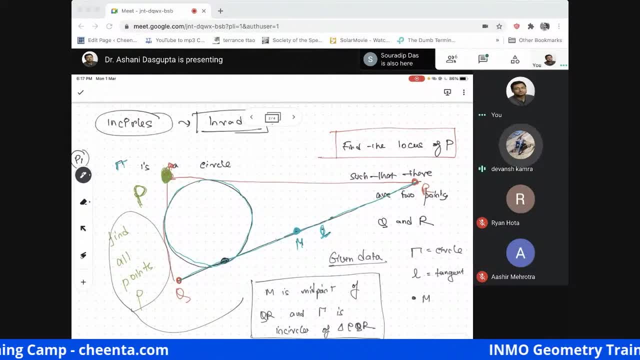 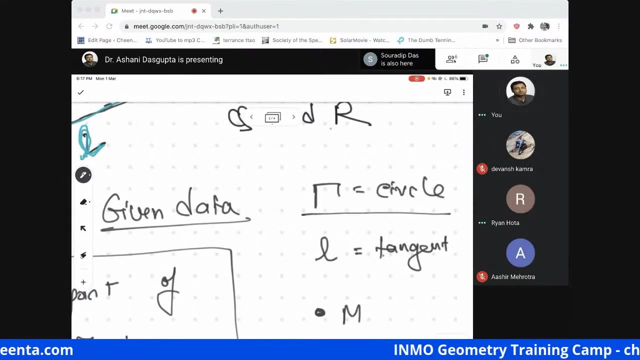 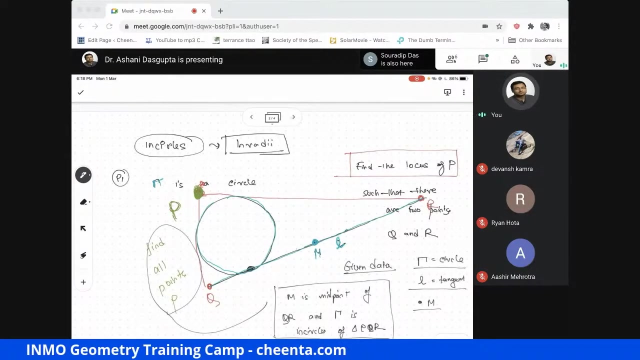 equation can be written as: X minus M square plus Y minus N square equals to N, where M and N are center for the circle. okay, what is the given thing? M and this is a given data gamma is given. L is given. M is given okay. okay. so what Devansh is suggesting is that we can. 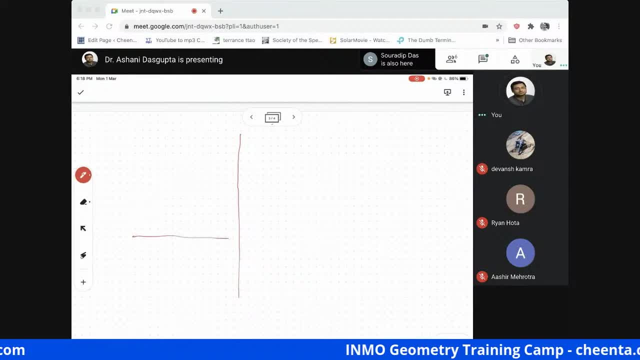 start with a coordinate plane and if we make things simpler, let's take this as a circle and let's take the X axis as the line L, M on the x-axis, M is a comma zero. let's take the Point M on the x-axis, so M is maybe. 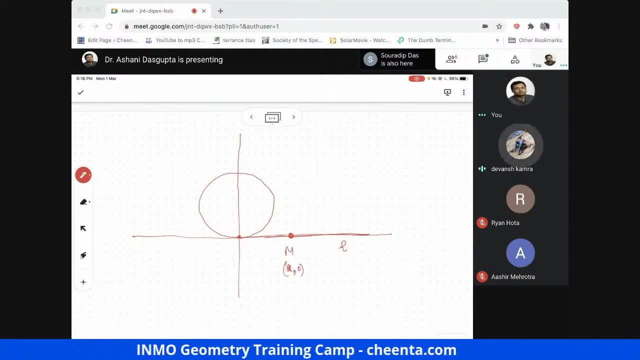 a comma-zero. yes, sir, I think it would be easier if you take M as the origin 0, comma 0 and the circle, or touching the x-axis at some other point. okay, so you are suggesting that you consider the point 0 as h, its reference point z as the origin point 0, and then options is called litex. 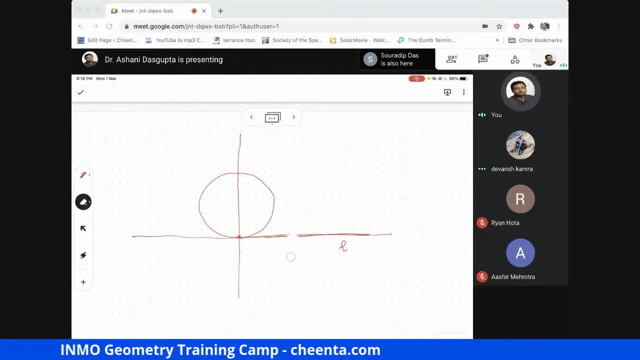 that. take the special case where m is the point of tangency. no, sir, take m to be origin and move the circle along the x-axis to some some point else. okay, i see, so do that. okay, okay, fine, maybe draw it like this. all right, now we can assume the center to be i comma j. let's assume the center to be i comma j. okay. 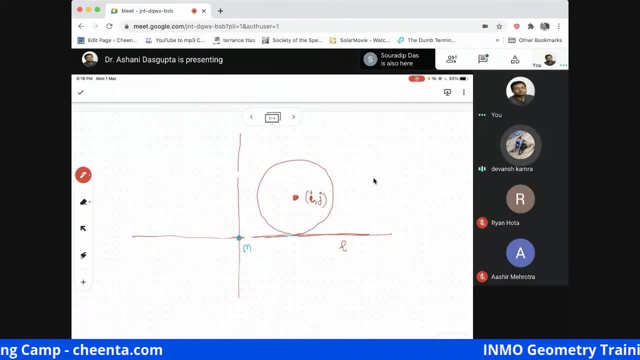 so we would have the equation of the circle x minus i square, i square. plus y minus j square equals to j. j squared, okay, equals to j square. okay, because j is the length of the radius. all right, and now, uh. now, sir, we know that the uh, i mean. 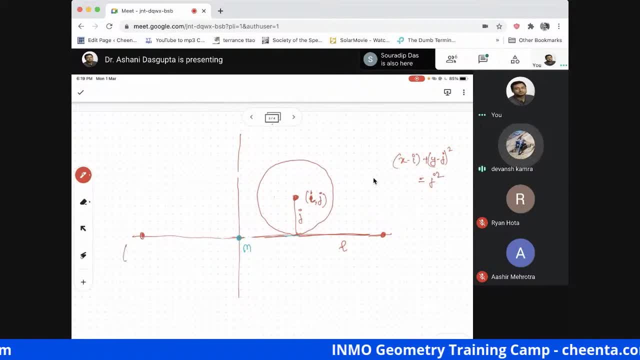 the points given down must be on the opposite ends of gamma. to make a make, a gamma is a inscribed circle. yeah, if m is the midpoint of, if m is the midpoint of this point of the circle, then the point of the circle is the midpoint of the circle. 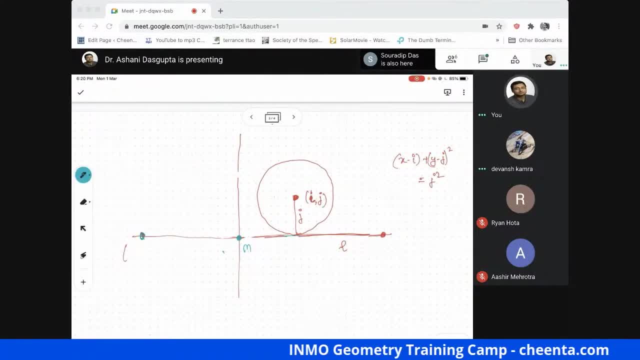 particular part, then certainly this is negative. a comma zero and this is a comma zero. okay, yes, sir, and p is the intersection of tangents. from these points, so we can find the equation of the tangents and find the uh, their intersection, which would give us an equation for p. 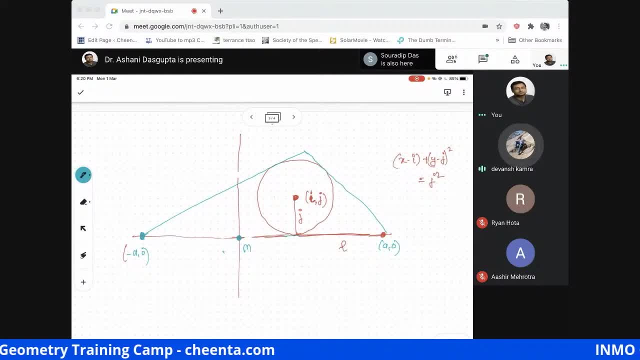 okay, let's do that. we can try to determine the locus from that. okay, that's very good. actually, why don't you, uh, why don't you try that? what is so? there is this equation of a tangent, equation of a tangent to a circle. so i think all of you know this, maybe i i also kind of forgot it. let's see, there is this. 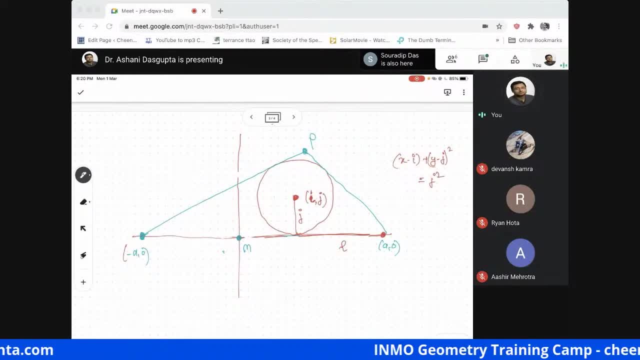 central. there is a general form of an equation where you just replace one of the values by the other one. so what you do is: let's see, uh, if we have an equation of a tangent to a circle, let's say we have an equation like this: x square plus y square plus 2, g, x plus 2, f, y plus c, equal to 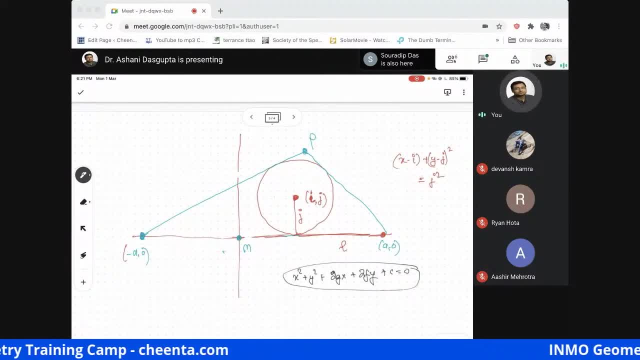 0. if this is the equation of a circle, then the equation of a tangent to the circle is given by x, x, 1 plus y, y, 1 plus 2, g, x plus x, 1 plus 2, f, y plus y, 1 plus c, equal to 0.. so this is the. this is a general form of a tangent equation, so now you can try to figure it out. give it a try. all of you try to finish the so. 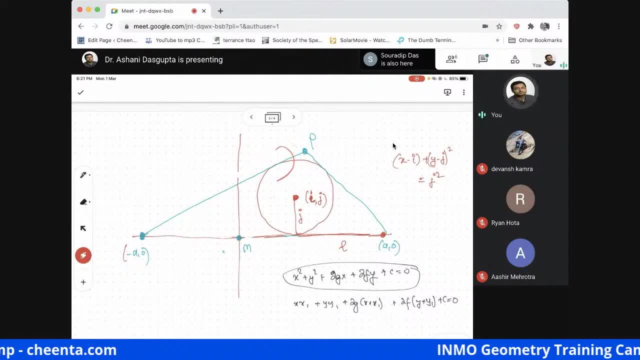 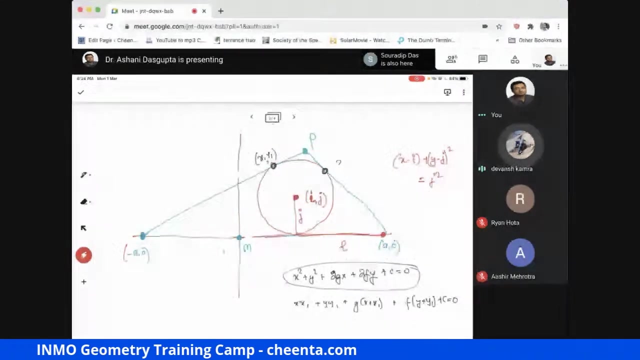 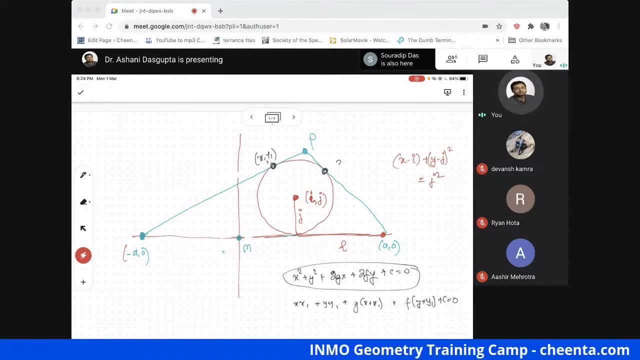 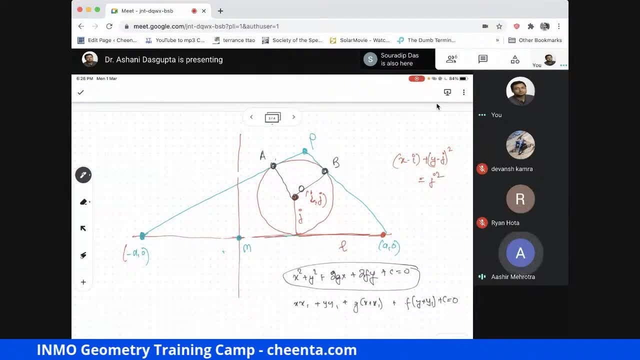 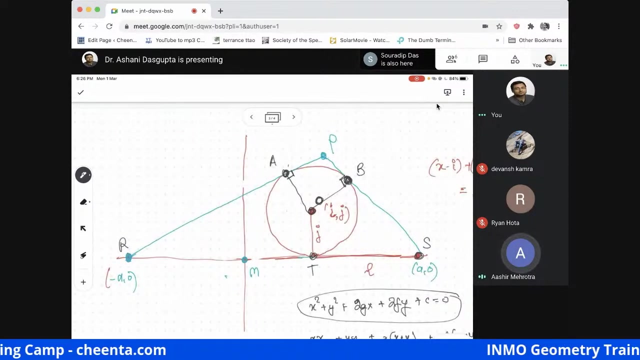 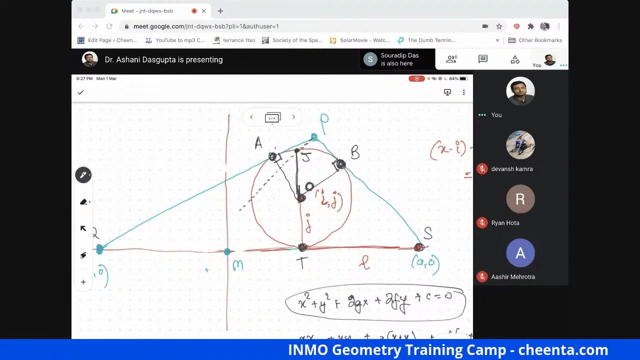 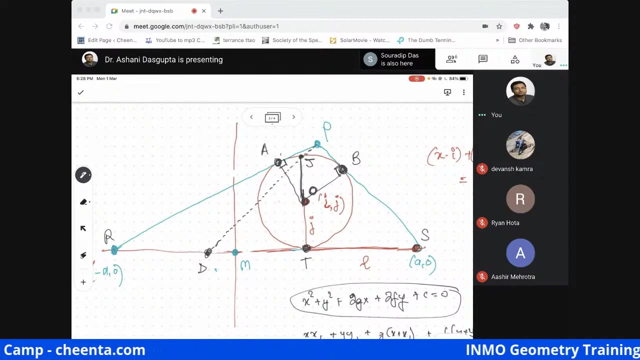 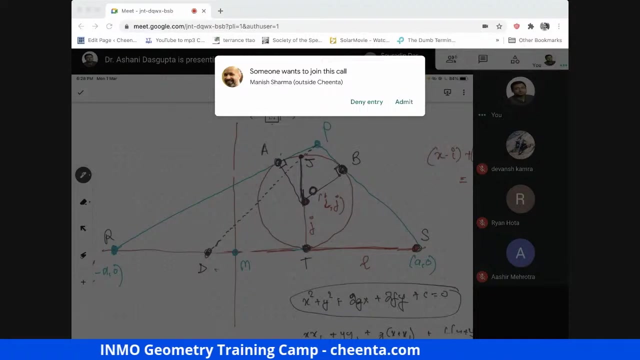 Thank you, Thank you, Thank you. So what can we say about PJ? So I just extend PJ to the point D. Suppose we don't have D yet, right, Extend PJ to D Then. Oh, someone else is trying to enter. 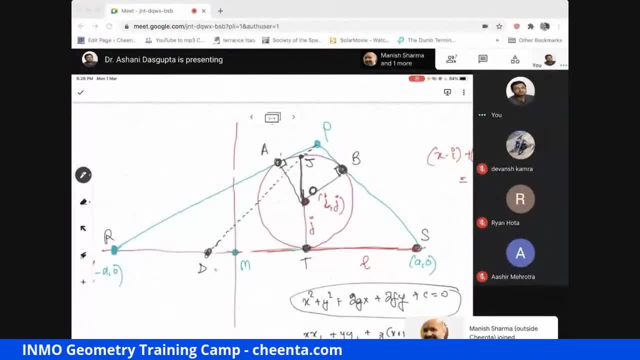 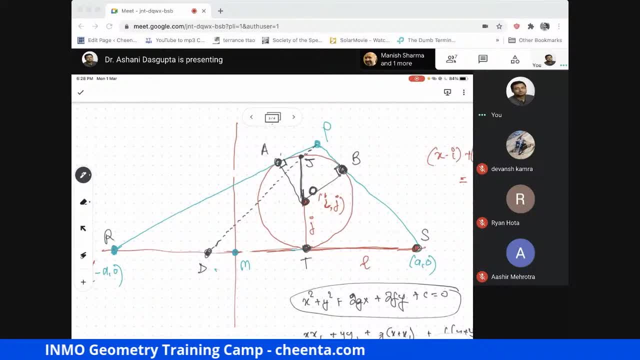 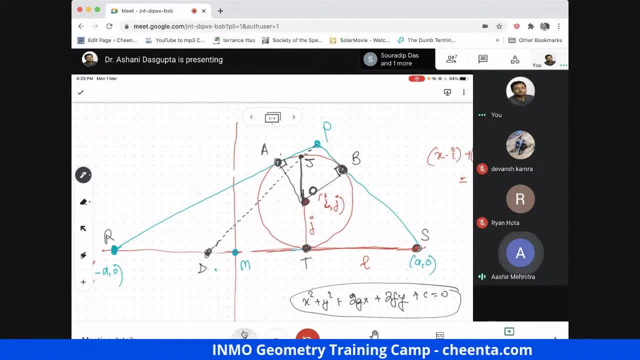 So we have got an L, An L, so using that we can find a. i mean, we'll find the line which a passes. i think we'll find the tangent line. oh, you can find the line in the sense, this line. yeah, so because r, a is perpendicular to a o. 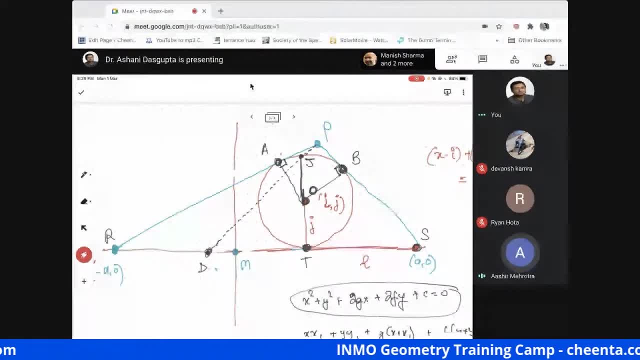 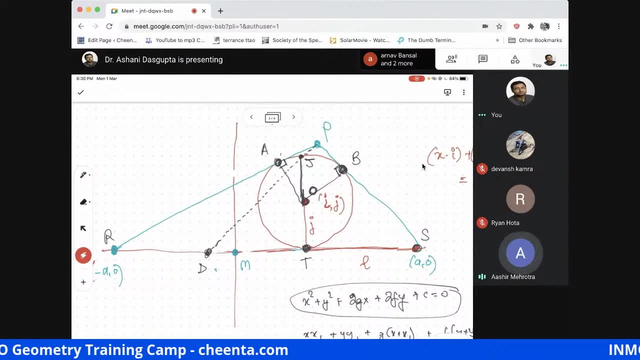 so i, using vectors, you know dot product thing. okay, wait, but basically let's say a is a1, comma, a2 sir. yes, sir, would finding the coordinates for the point d help? yes, also because i think so we can find the coordinates of a. uh, point d, sir. there was a theorem called, there was a lemma, sir, like 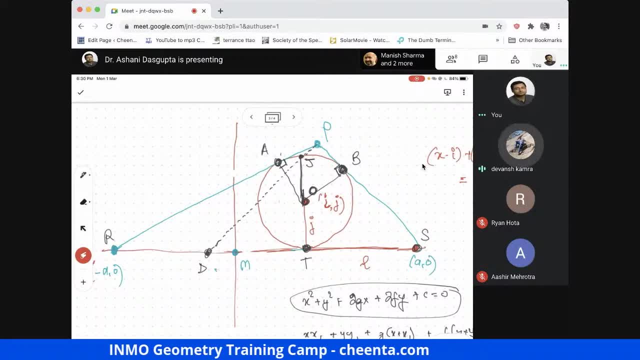 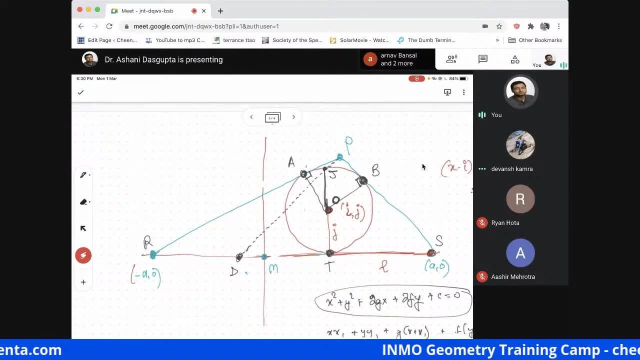 called diameter of the in circle lemma. okay, to that lemma. rd and ts are equal, sir. rd and d? ds. you know, rd and uh. if i remember properly, sir, then rd and ts were equal. yeah, you mean that d and m are same points? no, sir, sir, rd and ts are equal. rd and ts are equal, okay, yeah, of course. 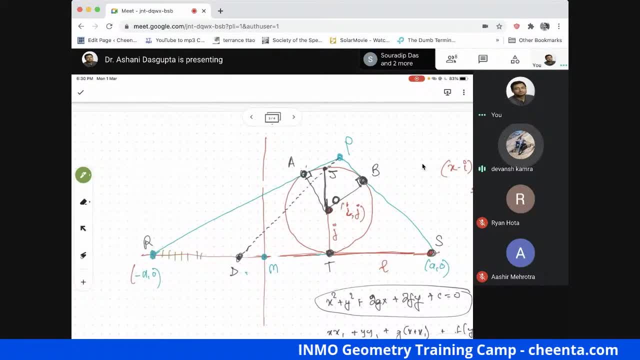 why is that? i said there was a lemma called diameter of the insert, lemma sir. okay, according to that, it was given that, lemma sir. i don't properly remember the proof. sir, for that you're right. we're actually using that here. so can all of you first prove that rd? 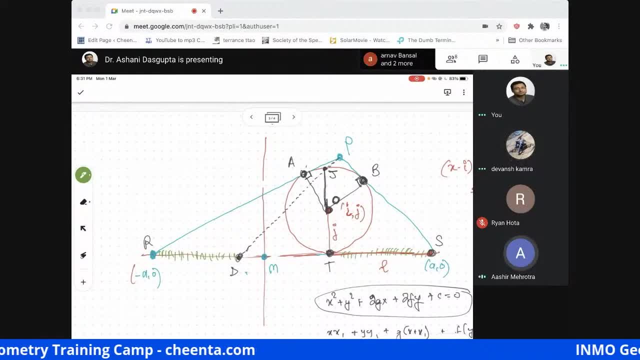 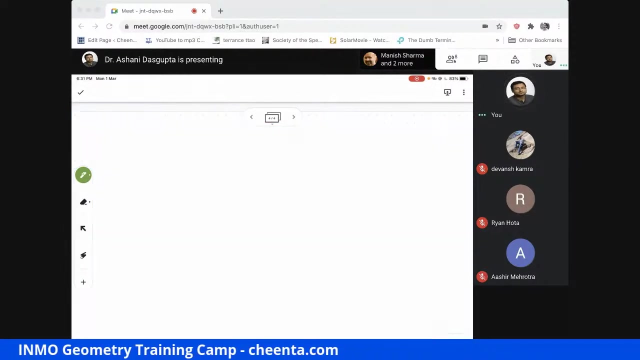 equal to ds. oh, i just checked it out because this will be one of the key tools of what we are trying to do. so can you prove that rd is equal to ts? so what was? what is the story? the story is this: that if you have a triangle, abc. 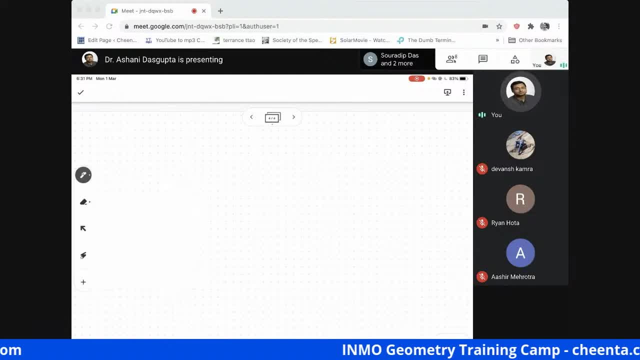 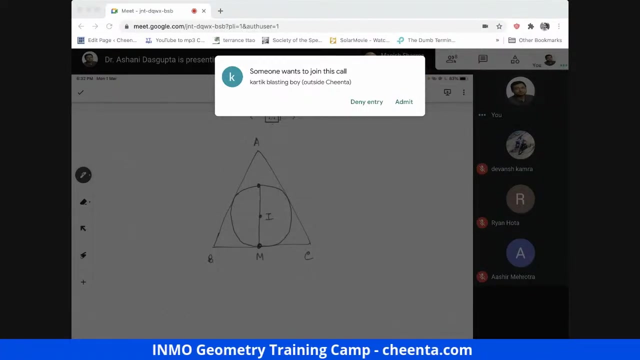 have a triangle abc. it's a very simple picture actually. if you have a triangle ABC and if you draw the in circle of this triangle like this, and if the point of tangency is M- suppose I is the center- and you extend the diameter to the point n, okay this. 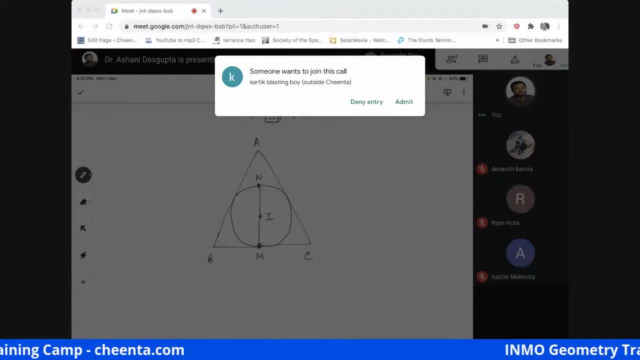 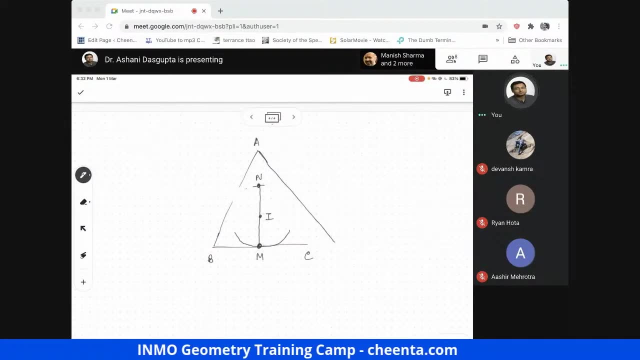 looks like like an isosceles triangle, so maybe to make it a little bit interesting, I have to make it a non isosceles triangle. so here we go, you have this circle, and okay, so this one is the point M. this is I, the in. 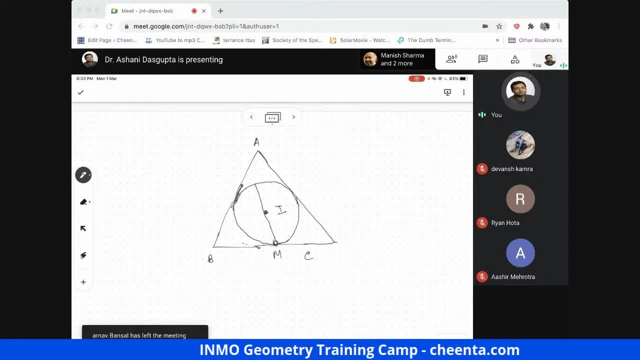 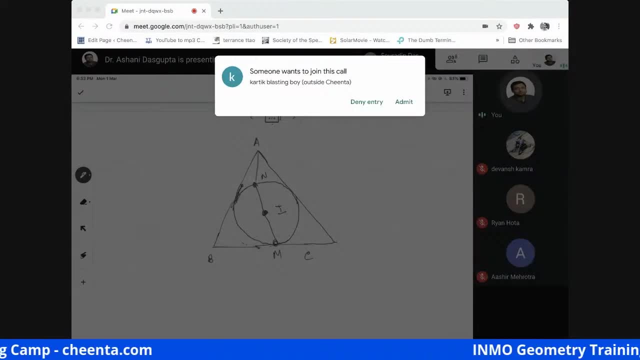 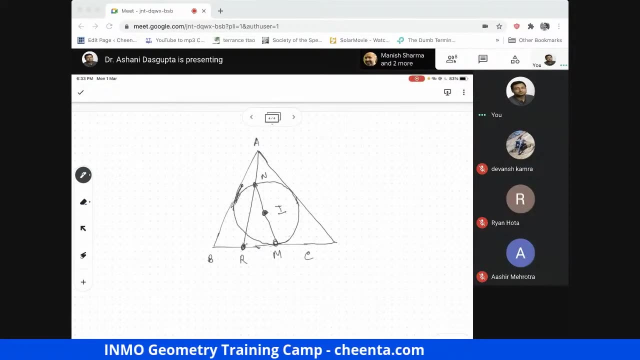 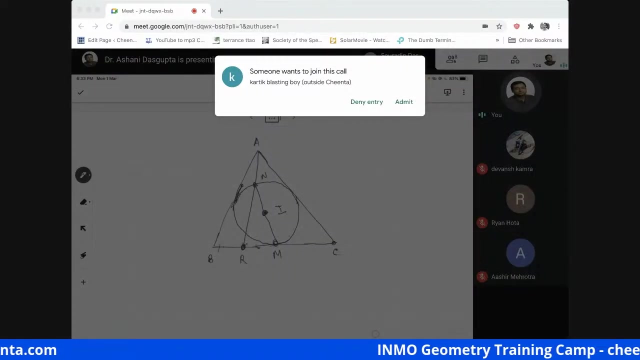 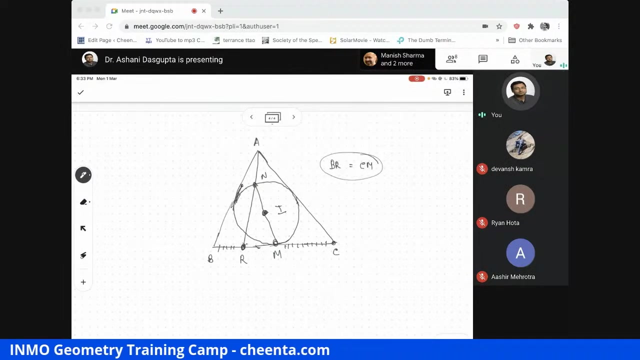 center and maybe I can draw it like this: M? n, we just draw the diameter and I will join a n to meet the opposite side. at the point R say BC. so we want to show that VR is equals to CM. all of the things that we are going to do. 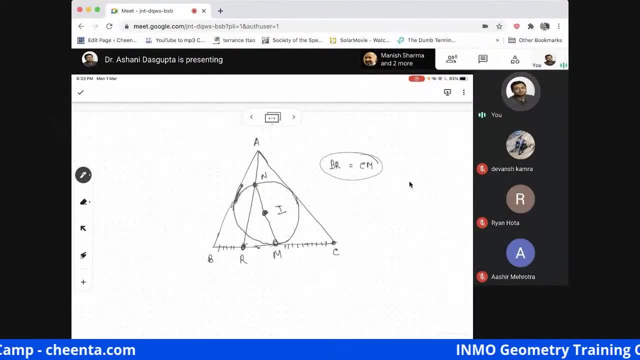 today will involve some fashion of this particular theorem. so can all of you try to prove this first? yes, so trying, just give us some time. yeah, yeah, and Devon, she's absolutely right, this is the diameter of in circle theorem. it's actually a limb, I mean, it's called. I would have in circle lemon. yeah, okay. 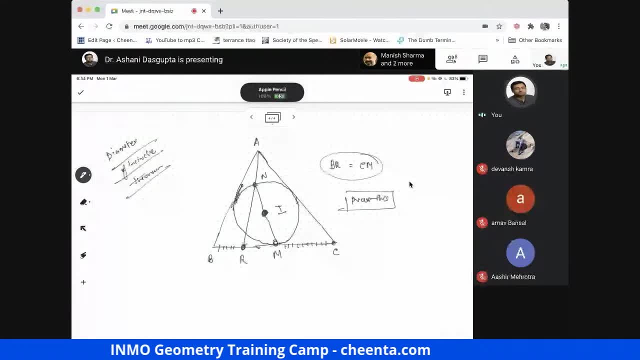 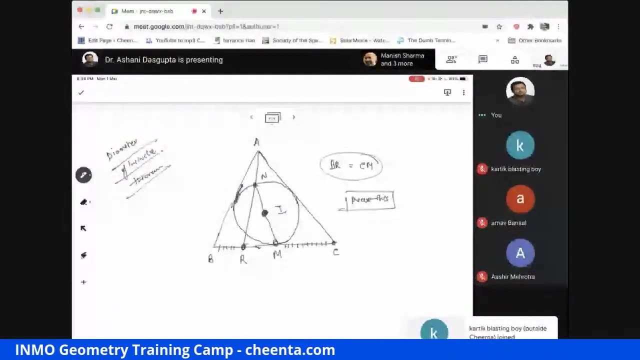 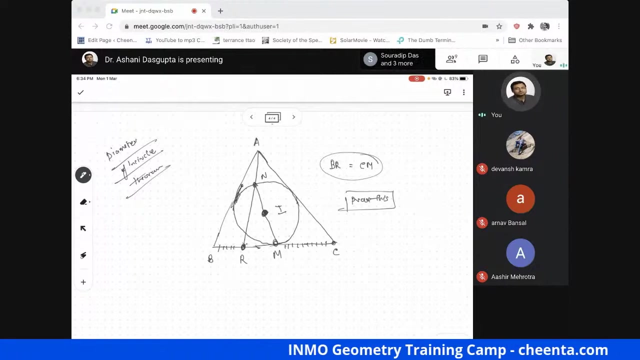 it's yeah, okay, let me get the power cord. I think I'm out of power already. just a second, okay, I think I'm almost out of power. just a second. you, I don't know how to tell you guys. can you mind showing me your hands? 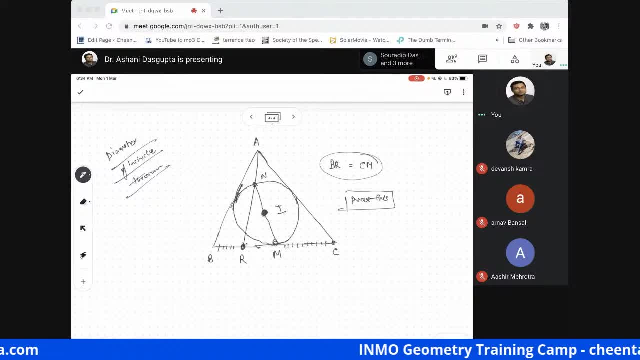 you don't have to turn the back off at all, but it does make a lot of sense to kind of show, if you do that, how far you can go into the direction of the direction of the power, and so that's why it's very nice to show that you could. 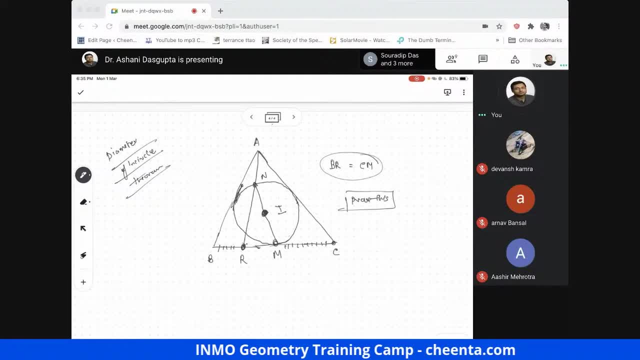 do that in a very similar way. line you obviously you know you could see a lot of different colors, but you could see a lot of the colors, but you could see a lot of the colors, but you could see a lot of the colors, and that's something I think. 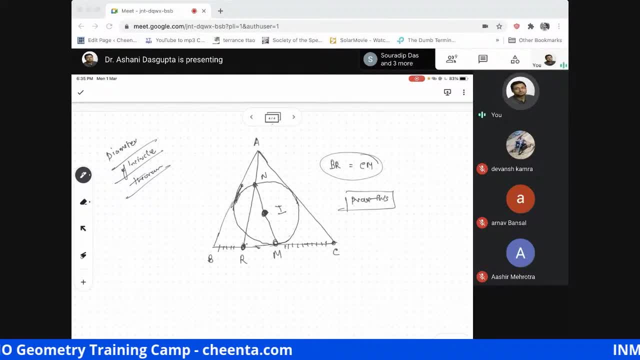 that you're very good at. you're doing a little bit better than I can, so I'm going to. OK, I'm almost out of charge, So I do have to take a minute, just a second. I got a proof, I think. 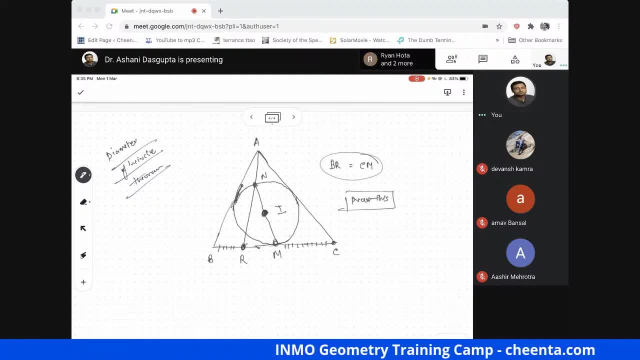 OK, go ahead. yes, You said you have a proof of this right. Yes, sort of I think. yeah, Basically we do homo 30 with center A, I think OK. And then we put it: OK, good, We can go to the x. Basically we make the in-circle go to the x-circle opposite. 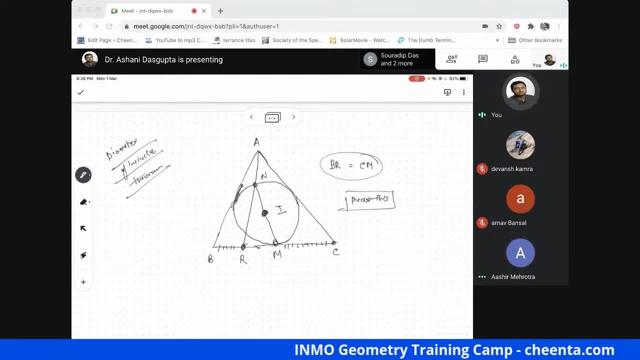 A x-circle opposite A. OK, that's interesting. The in-circle is maxed to the x-circle opposite A. OK, so let's extend this to. let's draw the x-circle. So the tangent point at BC will be R. 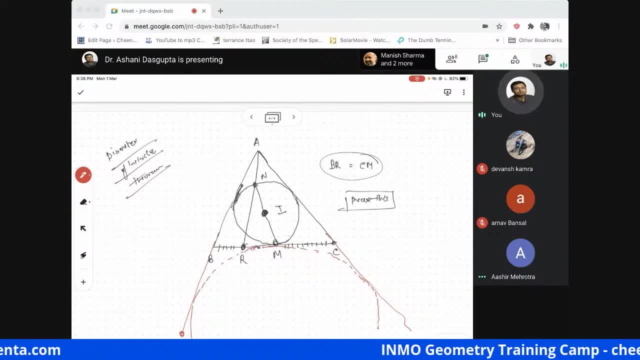 OK, So you're suggesting that this point right here will be this one. OK, Yeah, because of it, it's pretty obvious, because AN is wrapped right, Because sorry, sorry, M, So great, Let me just check. 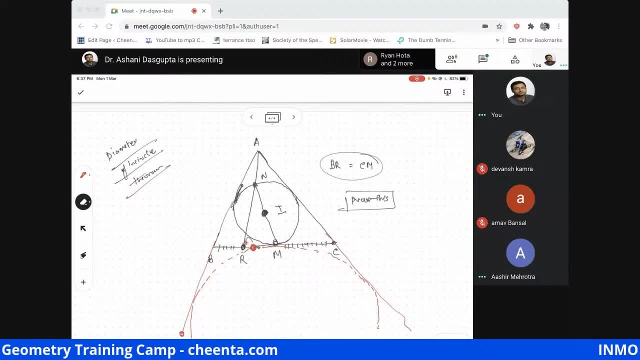 Yes, Sure, Take your time, But this is the. this is a very important tool. I mean, most of you know this. Yeah, because Yeah, What is the tangent like N is? maybe N is mapped to R right In the homothetate. 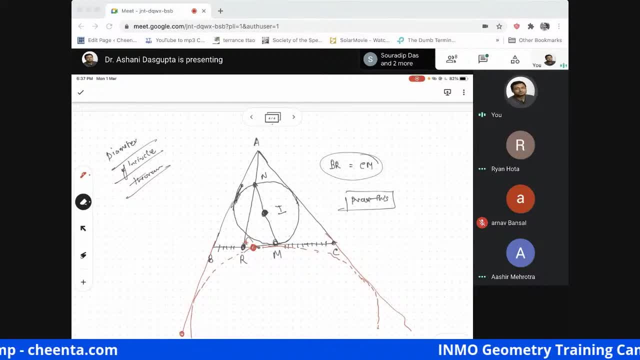 OK, so you were applying a homothetic about what? So A is the center of homothetic for you. Yeah, A is the center of homothetic. OK, A is the center of homothetic and you are mapping what to what. 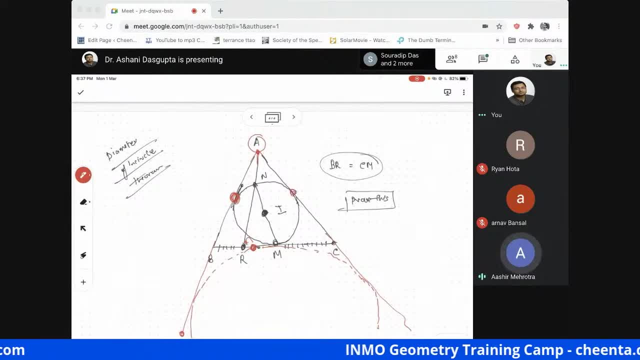 So I'm mapping the in-circle to the x-circle opposite. A, OK, that's fine. Yeah, okay, that's fantastic. so why do you think that can be done? what it obviously can be done? um, because, um, basically, if you look at a tangent point, you can, just if you, when you apply homo 30, it can. 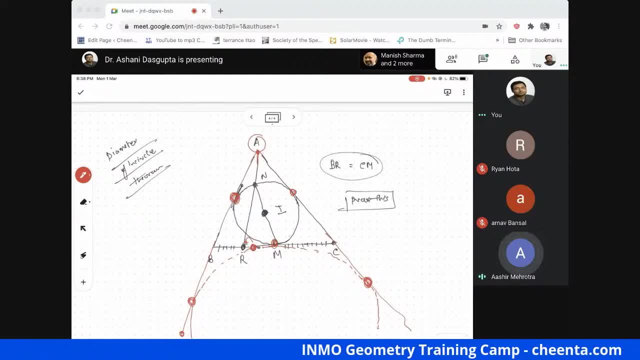 either go anywhere in that line, so we just okay. so basically yeah, so, um, yeah, sure, so let's call it r. okay, i have already used okay, x and y and z and w. okay, so you are suggesting that x. x goes to y. okay, x goes to z and y goes to w under the homo. 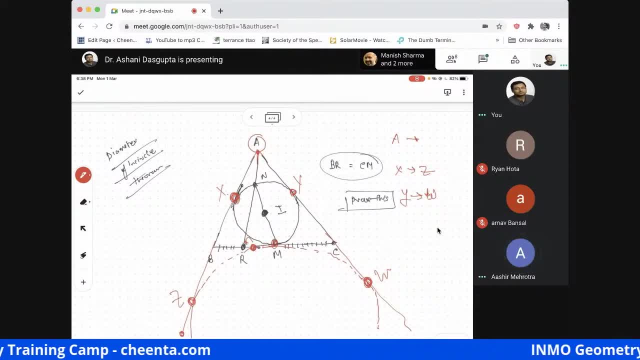 you got the ratio. so ax by ay is so ax by ay equals ax by ay equals a z by. let's do it, let's do it. isn't that obvious, as you say, dash it, that a x by a y is a very simple number. what is the value of x by a y? one one? 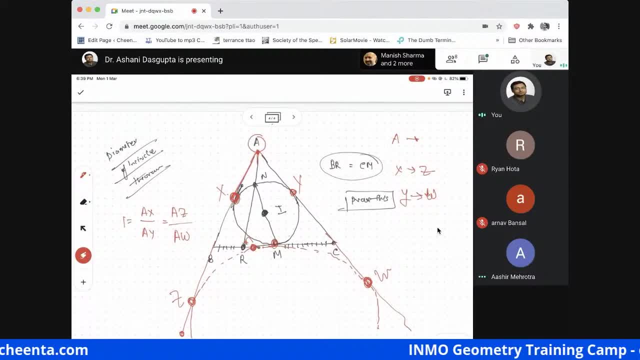 that's one right, because these are two tangents, two from a to the sag in circle, and a z by a w is certainly two tangents to the x circle from the point a. so so yeah, we get. we get that a x by a z equals a y by a w, so you can eat. so 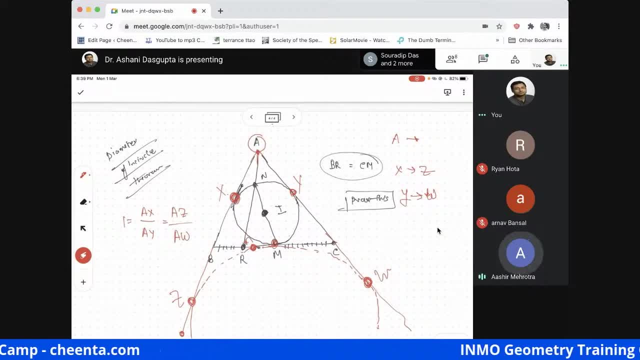 the map is actually justified. um, you can also do the same thing for the- yeah, for the third tangent point. so you know, yeah, something weird happens in the third tangent point. yeah, go ahead, you map those two tangent points to that and basically okay, just i, i, just i'm just curious, how would you? 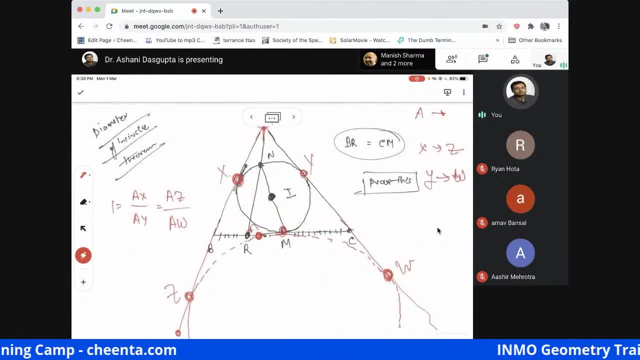 so, uh, okay, so then, then this particular circle gets mapped to. you are suggesting it gets mapped to this particular circle. yeah, okay, how is that? i mean, i mean that is true, but why would that be true? can we rigorously sort of talk about this sort of show? Yes, You are doing really well. I mean, this is fantastic. Yeah, so we need. 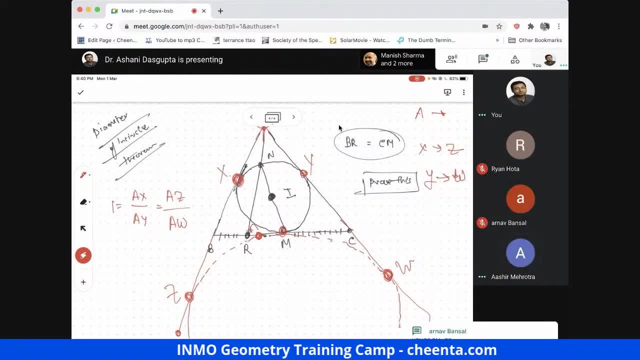 to just prove that the third time This is so good. So, those of you who are familiar with homothety, those of you who are familiar with homothety, I mean just let me, just, I should keep on trying. I'll just give a little. 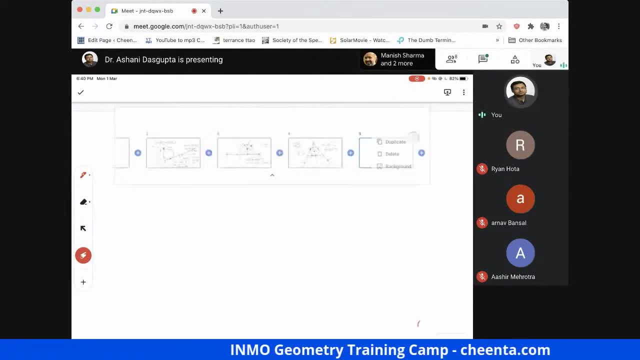 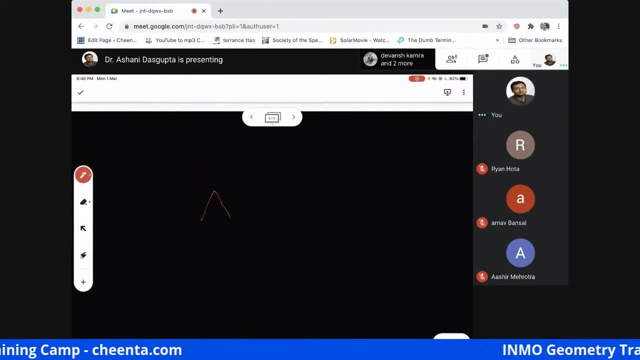 bit intro to people who are not familiar with homothety. It's very simple but very beautiful. This is it that if you have a triangle ABC, maybe I can draw it like this. If you have a triangle ABC And if you have a center called O, you may want. 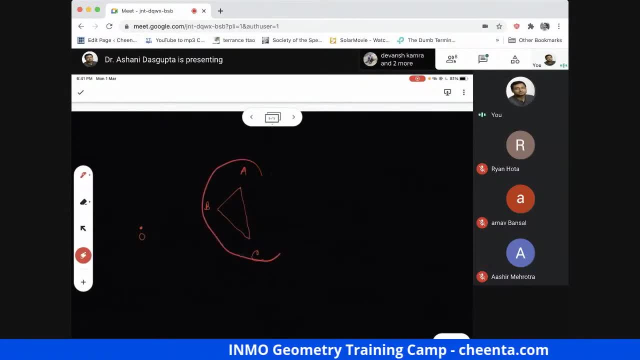 to blow up ABC. you want to, may want to blow up ABC into a larger triangle, or you may want to shrink down ABC into a smaller triangle. with respect to O, then O is known as the center of homothety. This transformation is known as homothety. So what you do is you connect and I'm saying: 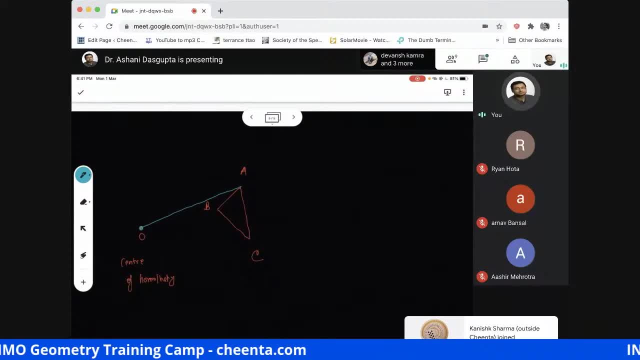 you want to blow it up. You want to blow it up. You may connect it like this, So like this, and the amount of like explosion or amount of expansion is kind is same, The ratio is same. So here we go. Here is a sort of a picture of the exploded version of ABC. 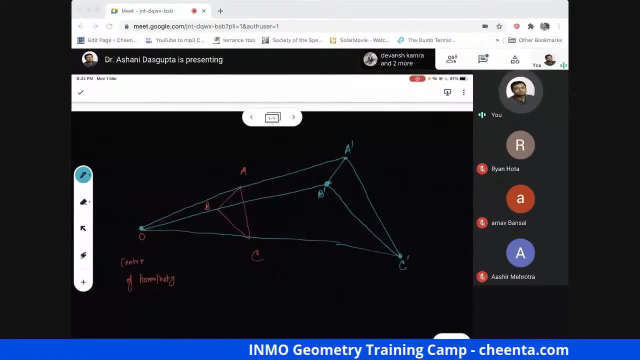 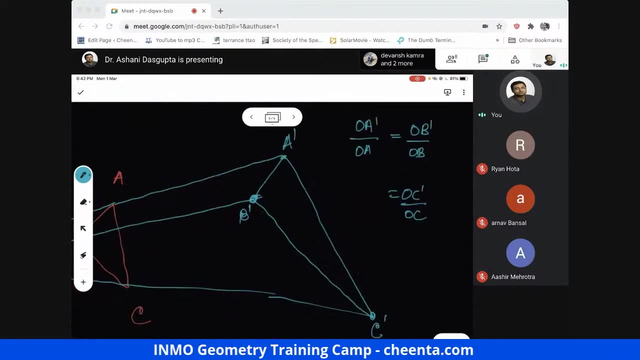 So when I say that they expand by the same amount, what I actually mean is that OA prime by OA is equal to OB. prime by OB is equal to OC prime by OC. Okay, so that's the meaning of when I say it gets expanded with respect to O. Now there, 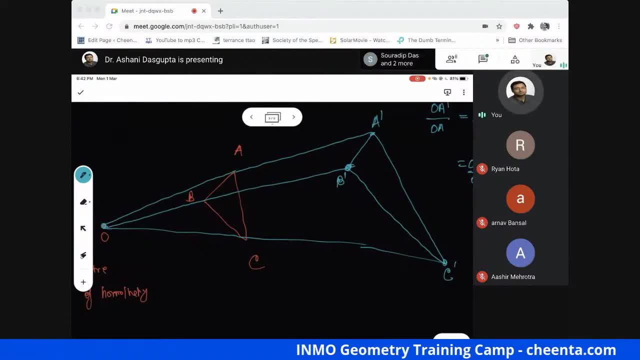 are a bunch of things that you can do when you are sorry. there's a bunch of things that you can do when you are doing homothety, For example. things that are in the same ratio remains in the same ratio. What do I mean by that? 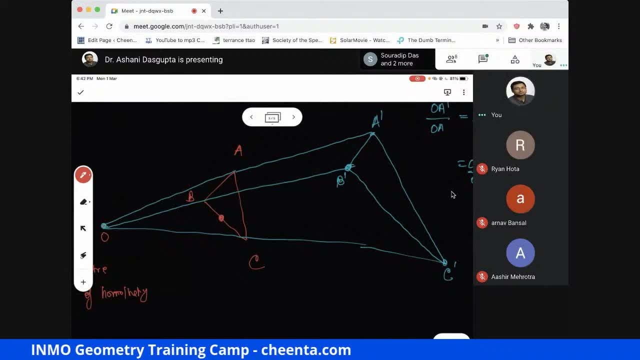 Well, if you take the midpoint of BC M, it would map to the midpoint of BC M prime. So I don't say that. I cannot say that if this is one unit away from B, If a point K is equal to A is one unit away from B, it will map to a point K one unit away from B. I cannot. 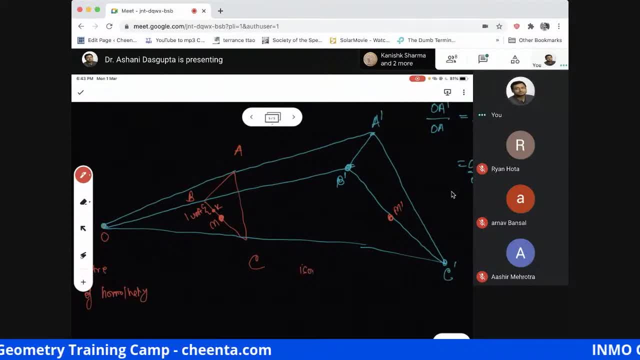 say that because that would mean isometry, that distances are preserved. So homothety is not necessarily an isometry, except for the identity homothety, I guess. But if you are looking at a non identity homothety, distances will not be preserved, ratios will. 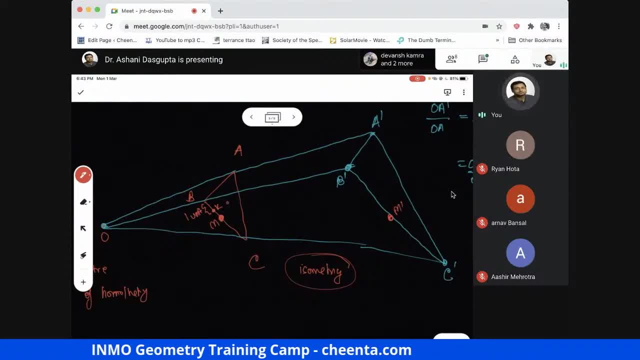 be preserved. For example, you can say that the centroid get maps to the centroid And an easy proof of this is that each of the midpoints will get mapped to the midpoints, Each of the midpoints will get mapped to the midpoints and the intersection of the midpoints. 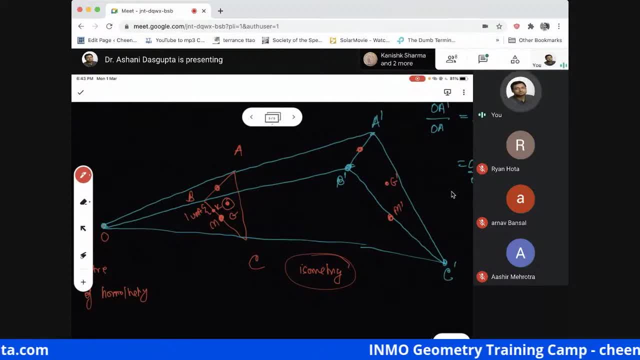 would be sort of mapped to each other. either you can say it like that or you can say, okay, this distance is one is to two. So it will be mapped to a point Which is which is at a distance one is to two which divides C n prime into one is to. 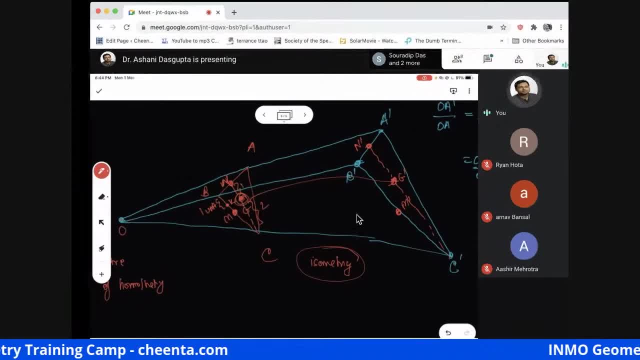 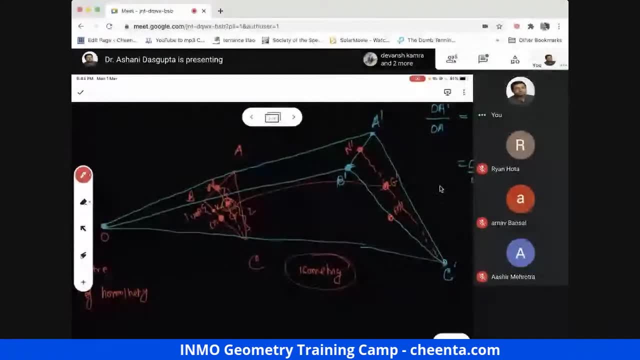 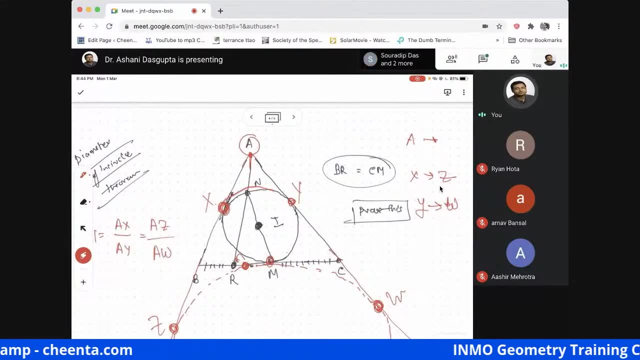 two, And we know that the centroid does that. So this is kind of easy, but it has. it has many beautiful properties. Now what here? what Arshad is suggesting is that if you perform a homothety on this particular circle, Or let's say, this is your center of homothety, center of homothety, and what you do is you 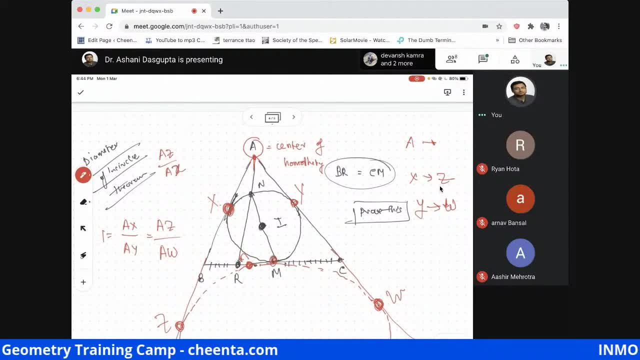 the ratio of homothety is AZ by AX. So you blow up by this much this ratio. maybe this is 2.9. I don't know what this value is, maybe it is 2.9.. So when I say that the ratio of homothety is 2.9.. 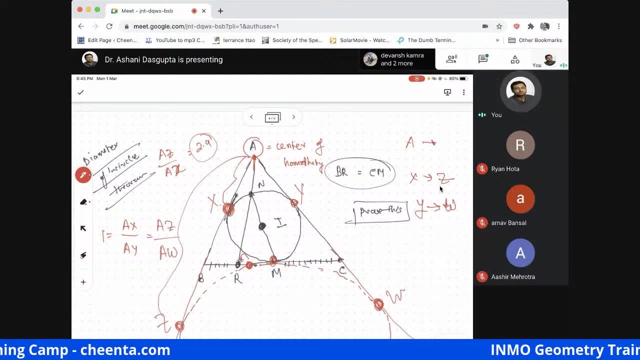 So you blow up by this much this ratio. maybe this is 2.9.. What I mean is you blow up everything 2.9 times every point out there. Okay, so this is what Arshad is suggesting, how she is doing here. 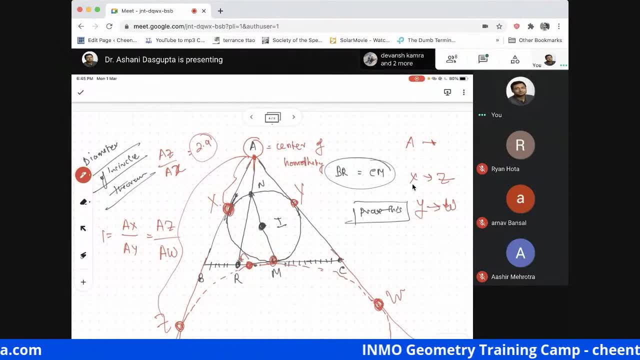 Now he is saying that under this homothety, M goes to. what are you saying? M goes to R. is that what you're saying, or? N goes to R? N goes to R, Okay. he is suggesting that N goes to R, Okay. 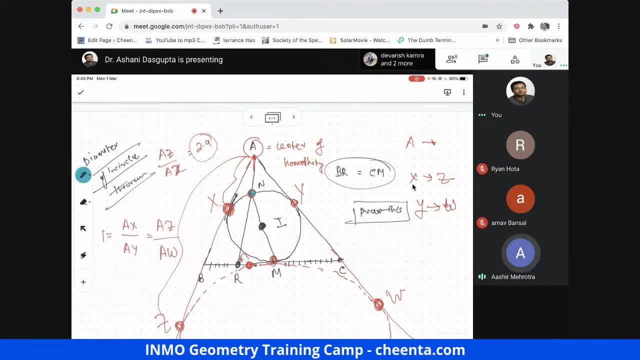 Let's define the homothety as N going to R. Okay, so if he has to prove that, then he has to show that AN by AR is equals to AX by AZ is equals to AY by AW. Okay, why would that be true? 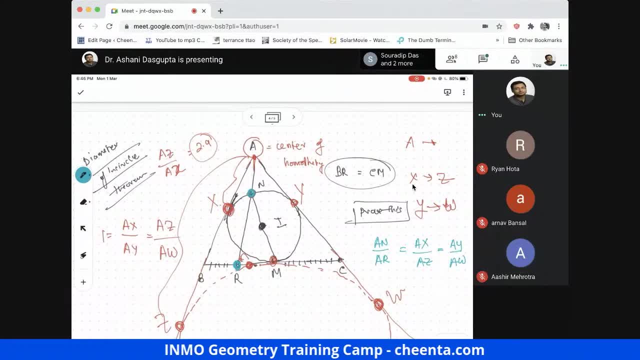 Okay, Okay, Because if that happens, something really really nice is going on here And we can say weird things, like in circles getting homothetized to X circles, right. That's why this particular lemma or theorem, whatever you say, is so powerful. 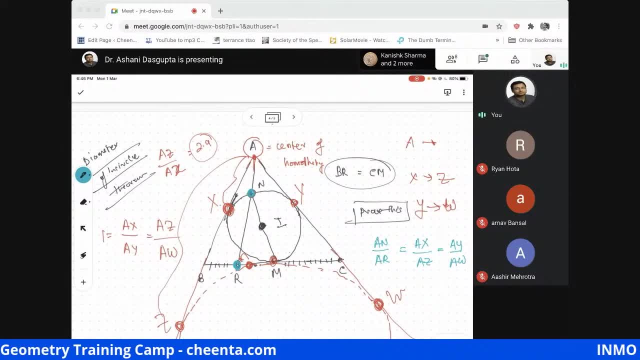 By synthetic geometry is nothing, it's just another problem, but it's actually something much more deep. Okay, Go ahead, please. I'm still thinking- Yeah, All of you try to prove this with Asher- that AN by AR is equals to AX by AZ, and so on. 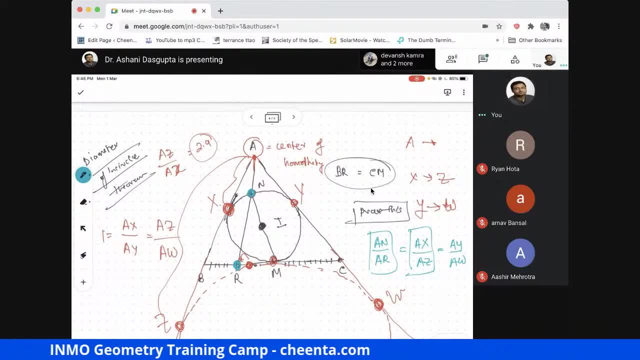 And you know I am very tempted to look at Google when I do this kind of problems, because of course this is a very old problem that solutions must be there in Google. But let's not do that, for today We're doing: 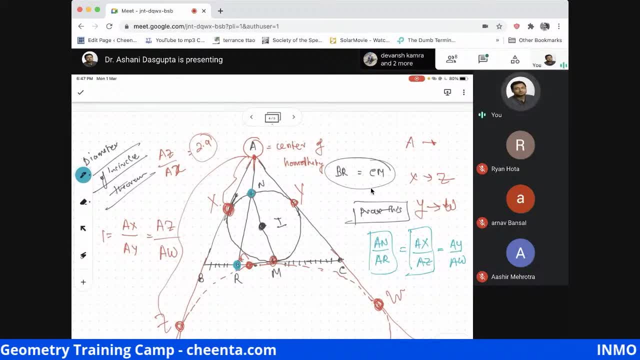 This is for fun, And I keep on forgetting all these proofs, So it's as if I'm doing it for the first time. So no worries, just let's try this And this, this can be. this is this should be doable. 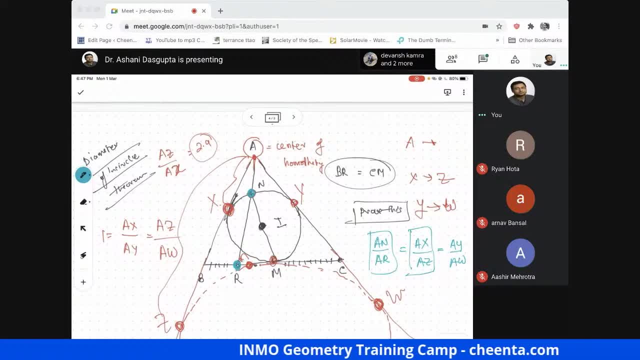 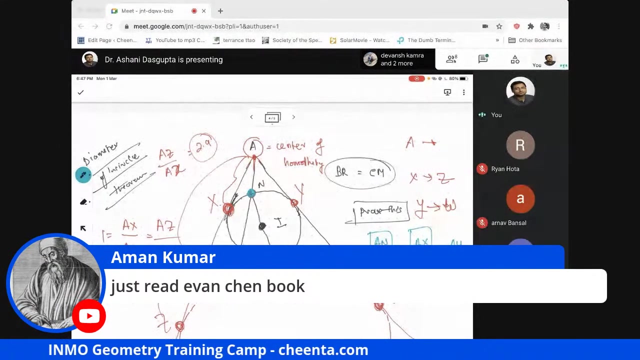 Okay, Okay. By the way, in YouTube I see that one student, a man Kumar, is suggesting that you should read the event Shела book. I think it's a very good suggestion, You guys, You Guys, if you are not using Ivan Shen's book on geometry. 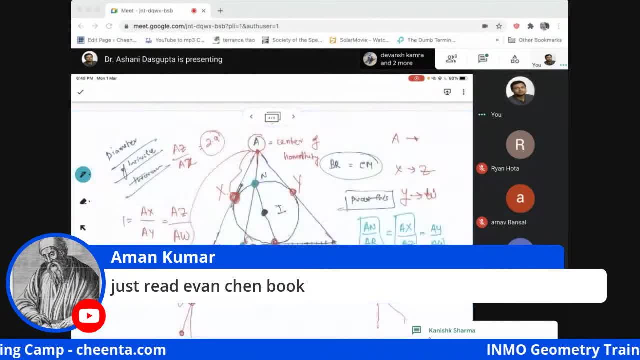 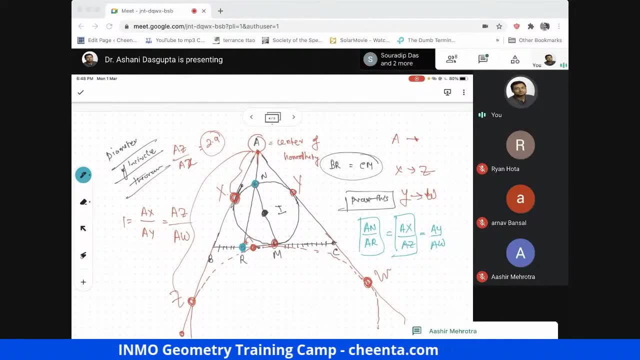 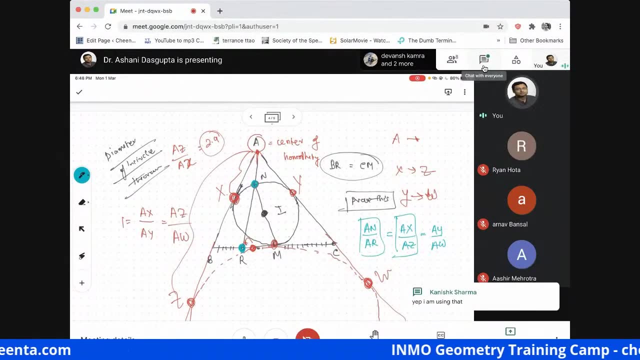 you should definitely use that. It's a very, very good piece of work, especially for Olympiad geometry. But I would also suggest that there are some other books on geometric transformation, especially Yaglom. I would strongly suggest Yaglom. 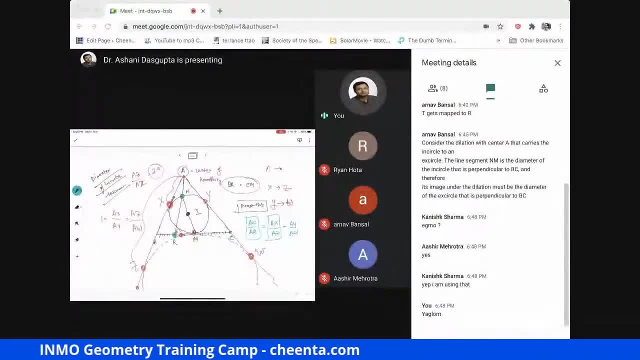 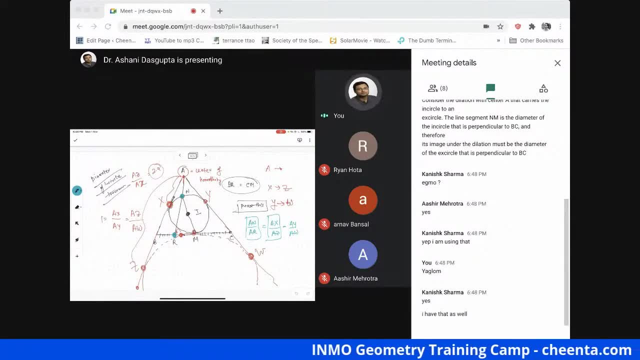 It's a very good book. Geometry Transformations, Part 1,, Part 2,, Part 3,, Part 4.. And 3 and 4,, I think, has homothetic and inversion, which are when I was learning some of these things. 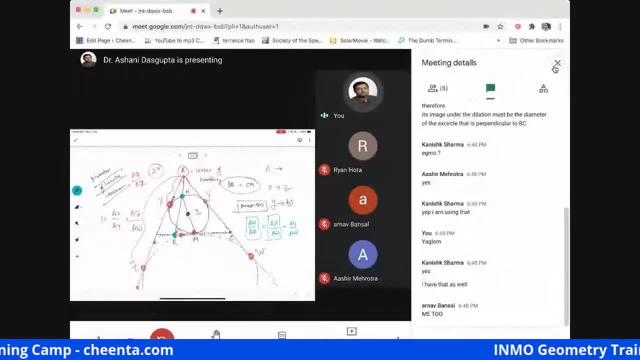 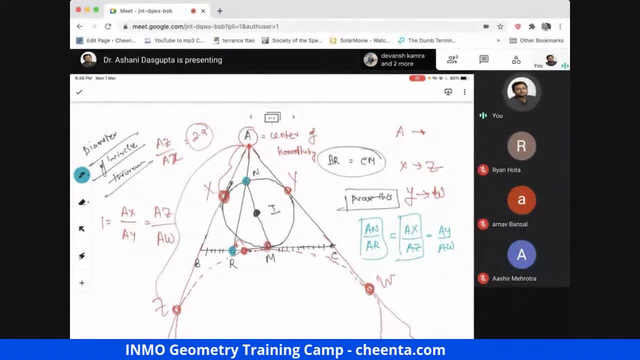 I did not use Ivan Shen's book. Honestly, I was using Yaglom to learn all of these, And he has a different style. It's a very nice kind of But, yeah sure, Ivan Shen's book is very nice as well. 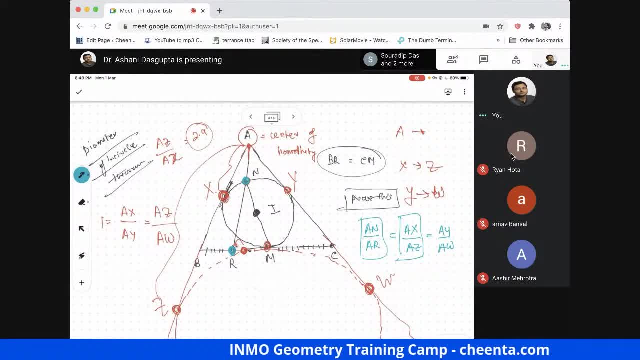 Hang on. So the question remains that if M is the center or is the point of tangency of the encircle and if N is the other of that diameter, if you join AN to R to meet BC at R, why would AN work out at far and if N was? 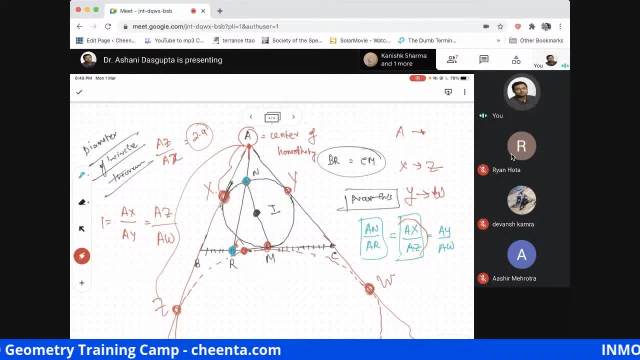 Y by ar be equal to ax by z. why would that happen? i mean, why would xn be parallel to zr? you see, if that happens, then xn will, xn will be parallel to zr, right, xn would be parallel to zr. why would that happen? 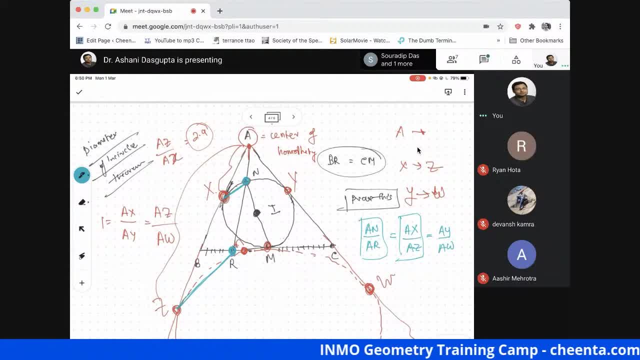 hello. so how about showing that x and a equals z r and x and a is equals to z r a? okay, okay, hmm, yeah, sorry, sir, does r lie on the x circle as of today? as of now, we don't know that. um r lies on the bc. right r lies on bc. yes, that we know. 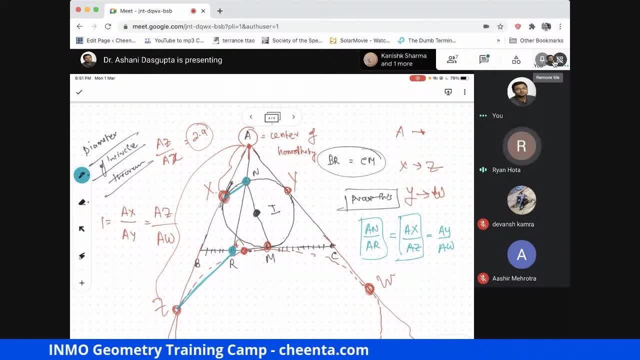 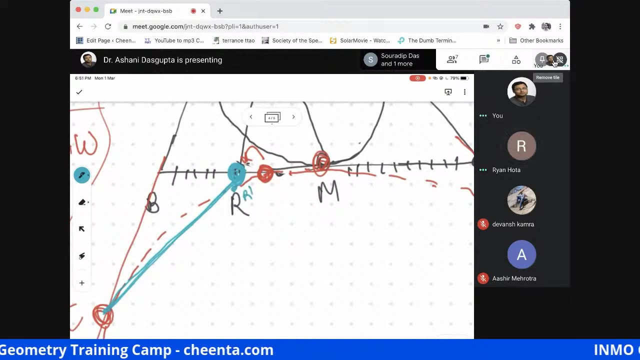 so my question is that, sir, if, if i extended, if i extended ar and made a point, r dash that lies on the x circle, okay, then it would, then it would appear that a n, x and a r dash, a r dash, c, a r dash, whatever. that point is just a second. let me. 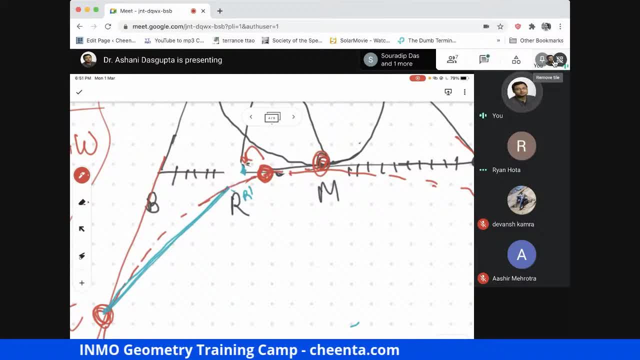 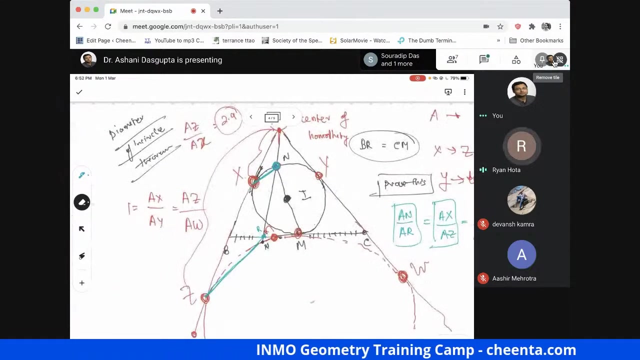 do what you are saying. first, you are saying that we are extending this thing to meet at a? r prime. okay, and there is this line: okay, here we go. this is the point. r okay, fine, and what did? what happens is that we can obviously prove that a a, n by a? r. 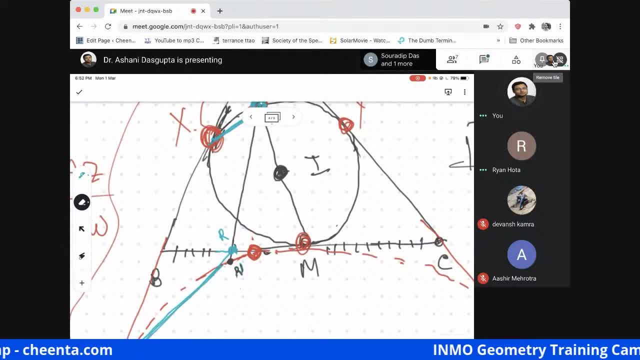 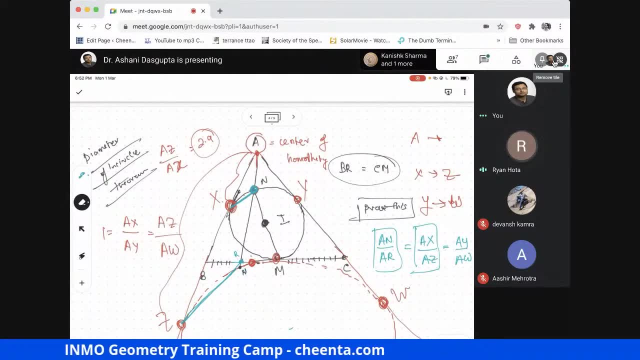 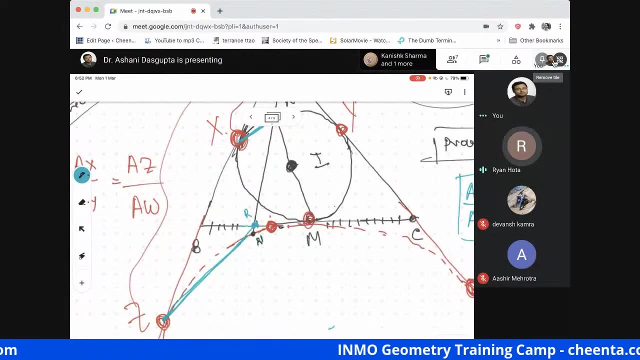 dash is equal to- please do not zoom in, sir- yeah, a n by a r dash that is equal to axz is equal to ax by az. why is that? because, sir, because we are basically what we are doing: we are expanding this circle. when we are going, when we are, we are going from in circle to x circle. when we 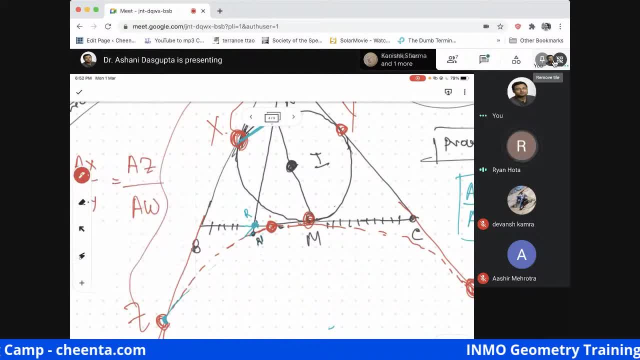 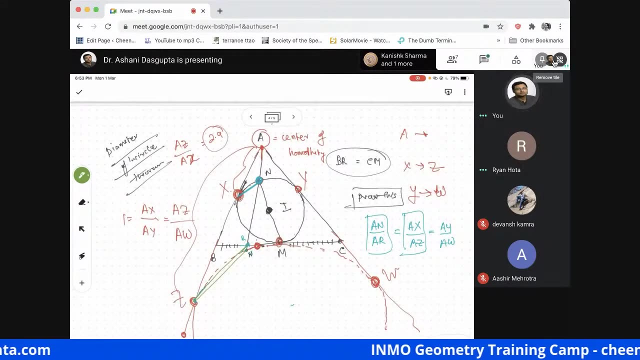 are expanding, when we are going from in circle to x circle, we are going from axn to azr, dash, dash, that okay. so now you are. now you what you are. okay, i would accept that, ryan, if you could show that a n by a r dashed is equal to a x by a z. you, either, you either tell me a reason why. 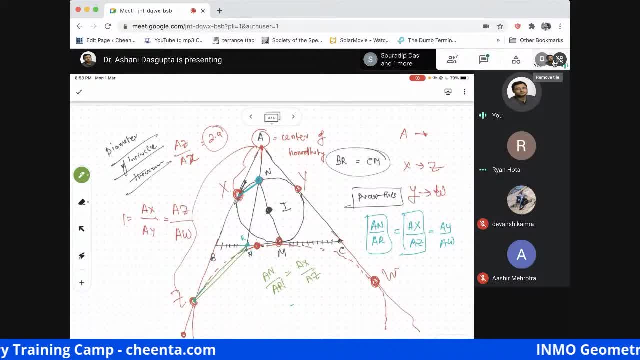 why a n? because i i don't believe, as of now, at this point, that this in circle is getting expanded to this uh other is to this x circle. so, and do you believe that the radius radius of in the in radius and x radius, the ratio of the in radius and x radius, is equal to ax by az? yeah, i. 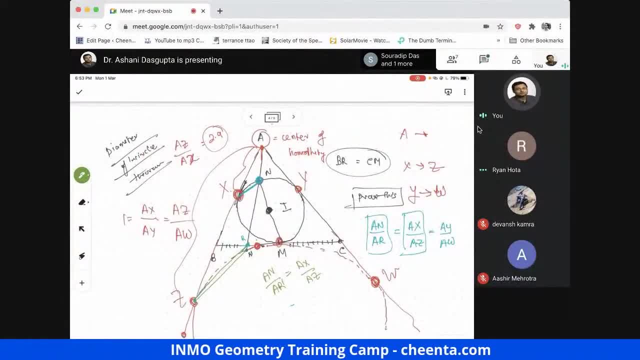 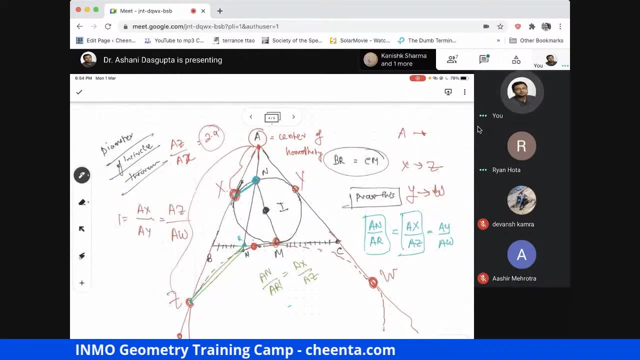 ninety percent believe it, because of course that would be: uh, can you, can you quickly show that? so, because if you, uh, what ai is the angular bisector? okay, i do believe that. let's say: since we are in an inmo camp, then we do believe that a, i, i, a. 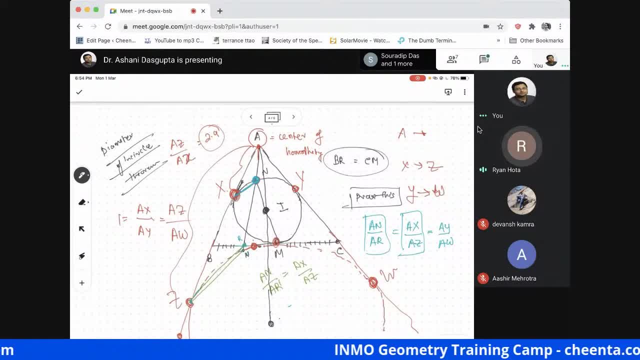 are in the same straight line. yes, sir. and then i x is a perpendicular, i a z is also perpendicular, and we get very simple, similar triangles. okay, i x is a perpendicular, so this is right angle. i a z is a right angle. so now, um, ryan has convinced me that i goes to. i a for sure. 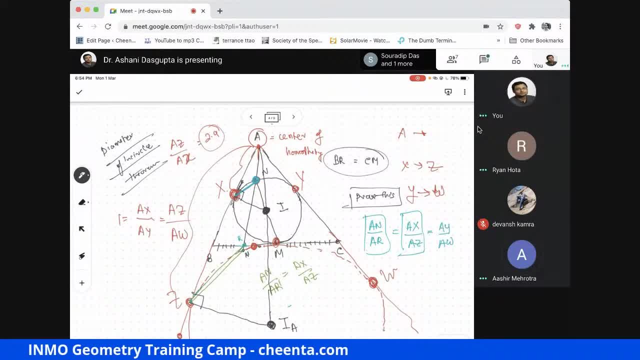 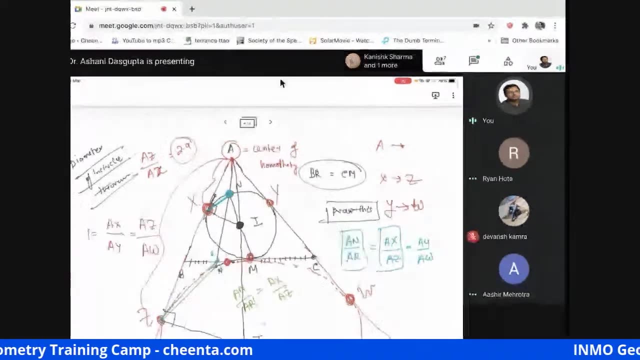 under the homogeneity. so i think we are almost done. no, we so we have. we have proved that the, the in center, sorry, the in circle- goes to the x circle. i think, well, we what we have proved. okay. so let's be very clear about what we have proved so far. we have proved that the center goes to the. 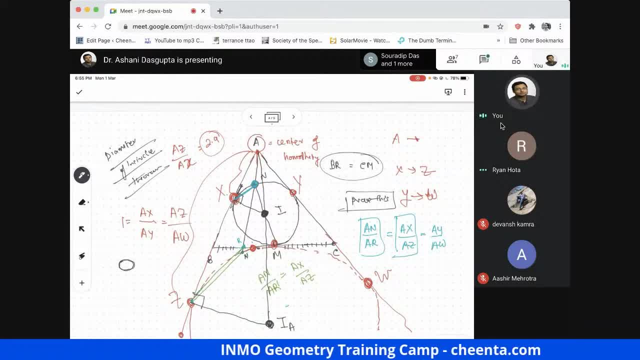 center. there are two circles. let's understand this carefully. there are two circles. we have showed that under homotheti, the center of one circle goes to the center of the other one. okay, we are happy about this much. we have also shown that the point of tangency x goes to the another point. okay. 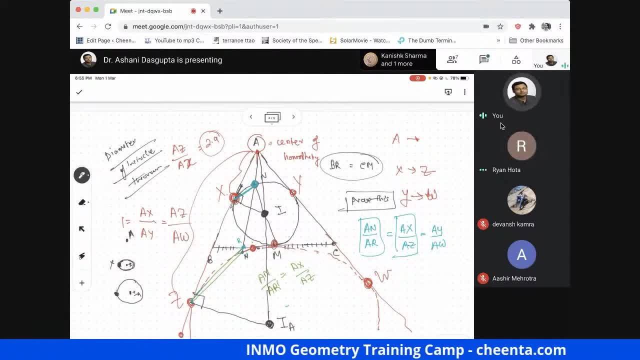 let's forget about the word tangency- and a point x goes to the point uh z and a point y goes to the point w under the same homotheti. let me ask you this: does that ensure that the circle goes to the circle? sir, i do not care whether it ensures, because i know that the radius will go to the radius. 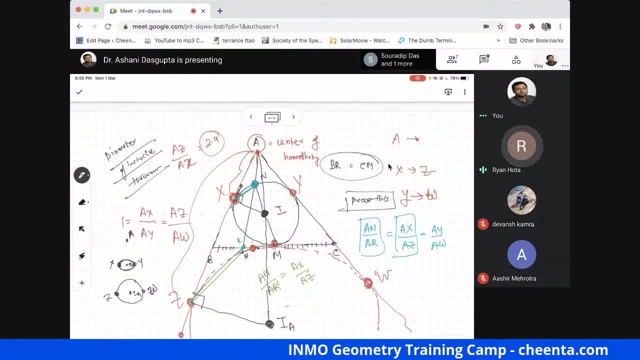 because the i, i, a x, i is similar to a z, i e, so i x will go to the i a z. okay, i do. i do concede that. okay, so this, definitely. so the ratio of radii and the ratio of the centers are equal, so i do not. 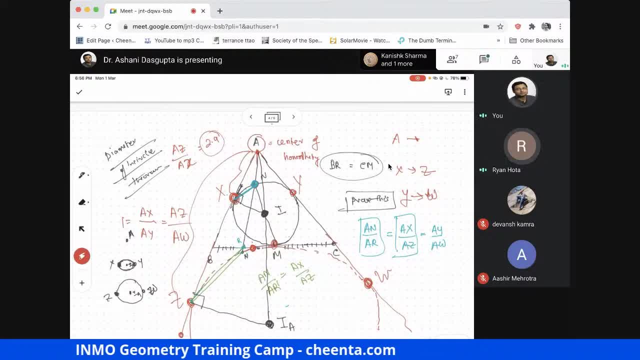 need to care about what x is and what z is, and okay, fine, that's, that's i. i accept your, your argument. that's very nice. so you are suggesting that the radius is going to the radius and the center is going to the center. that ensures that every point goes. 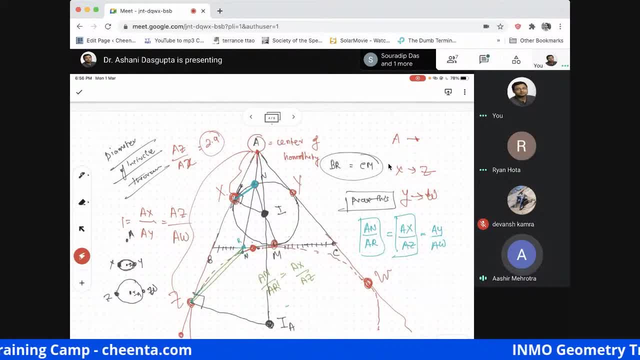 to the point, is going to open. we haven't proved that the center is going to the center, right? we do know that. right, because ai by aia is equal to ax by az, because these two triangles are similar. oh, yeah, yeah, so we know that center is going. so the center is going to the radius center. 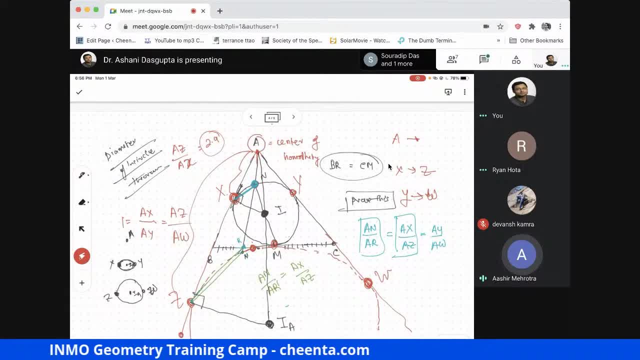 radius is going to the radius. why is that sorry? why is the radius going to the radius? because i x is equal to i a z, i a z. okay, is is sorry. i x by i a z, z is equal to a, i by a, i a a. but why is that? why is that okay? because of the similar triangle fact, right. 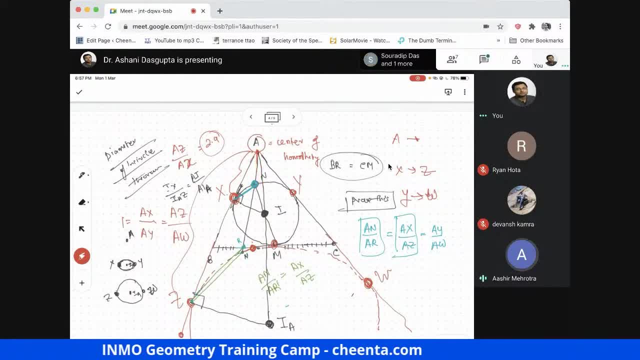 yeah, sorry, okay, yeah, so that we have proved it. sorry, we proved that the sar, so maybe, maybe, then maybe we prove that the circle in circle goes to the x circle. that's tremendous. there exists and there exists a, there exists a homothetic centered at a. 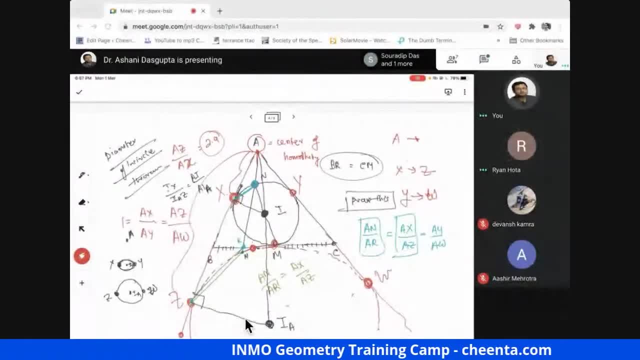 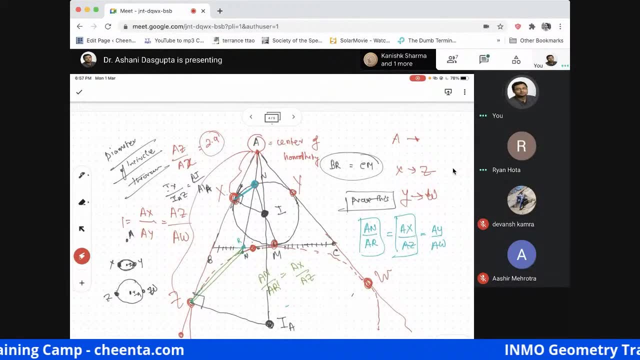 which sends the in circle to the x circle. we are very happy about this. but now the question is that clearly the point n is being sent to some point on this circle, r prime. so n is being sent to r prime now why would r prime lie on bc ryan was saying something about. 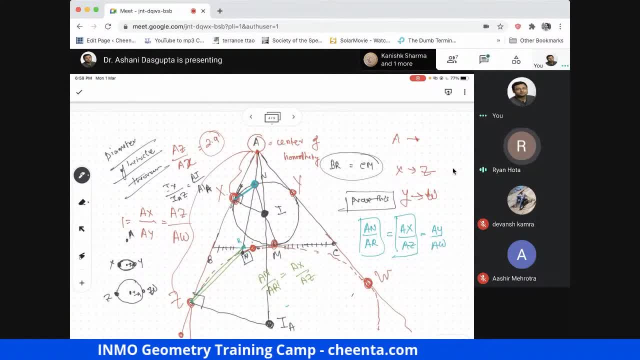 that. yes, sir, i do. i i guess a person's very unlikely, because we know can cases very unlikely to lie on bc. so maybe i thought there was a slight mistake in the what in the like in the statement. oh, maybe ryan is saying why is it on bc? maybe it is not on bc. 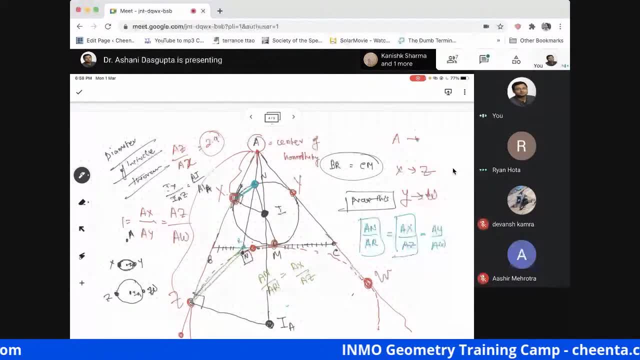 uh, okay, as of as of now, we don't have any evidence that r prime is always on bc. okay, i accept that. can anyone give me any evidence why it it would be on BC? we are trying to prove that r equals r prime. we are trying to. 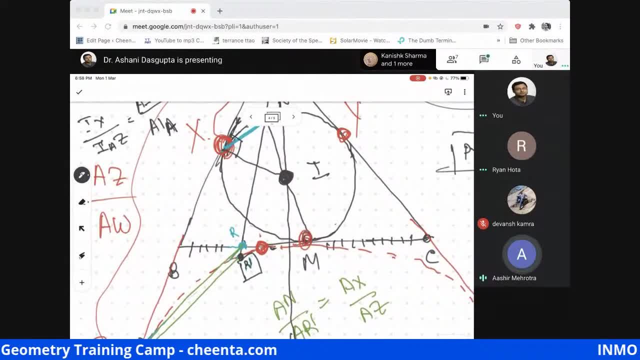 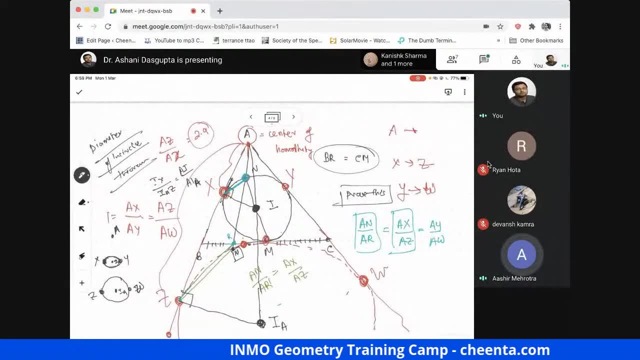 prove that r equals r prime, indeed. so wait, because yeah sure I can do that. so, and NM is a diameter, right? NM is indeed a diameter. yes, so it should be perpendicular to BC. nm is perpendicular to BC. yes, certainly, perpendicularity holds after homotheticity. homotheticity preserves angles because it's a. 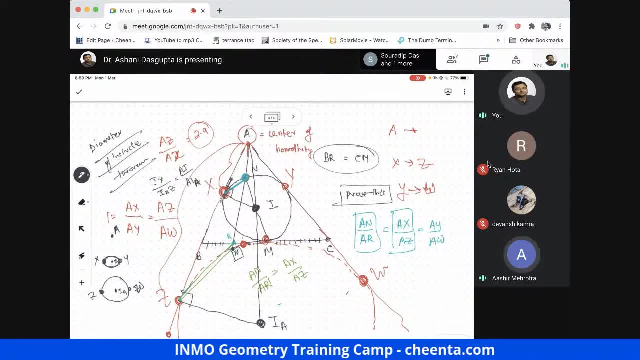 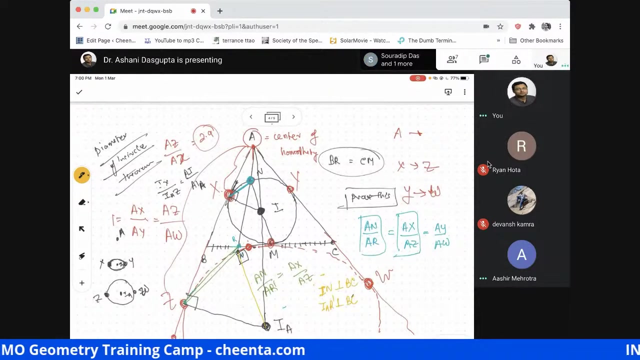 similarity transformation. so what Arshir is suggesting is- here is something fantastic: he's suggesting that I a are prime is perpendicular to BC. why? because it's pre-image MN, I, I, I n- sorry, I n- is perpendicular to BC. so I are not, I a, I a. I am not, I are prime, I a. are we okay I? 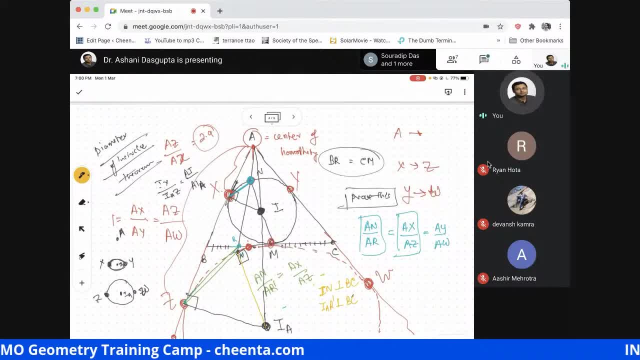 a are is perpendicular to BC. we know from a different fact that R is the point of tangency. so I a are is perpendicular to BC. this we know from the fact that this is a tangent, BC is a tangent. you know from the fact that this is a tangent, BC is a tangent, BC is a tangent. 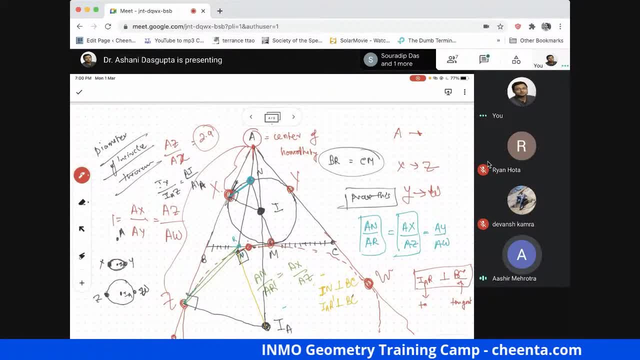 and not what of, but we don't know if our lies on the circle right. so, okay, I see what you're saying are you are and not to us, and I is not to I. okay, okay, okay, I think we need to sort of recalibrate a little bit, so let's let's forget about. 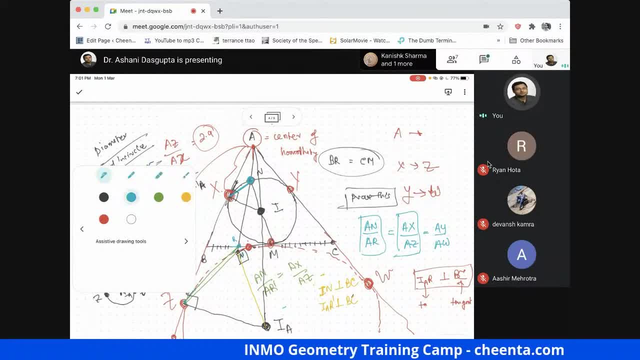 this point R. okay, instead of calling this one R, let's call this point as R, and I think that would be done. okay, so let's call this okay. okay, so now we will be done. can anyone give me a one line argument, by homogeneity, why I are? 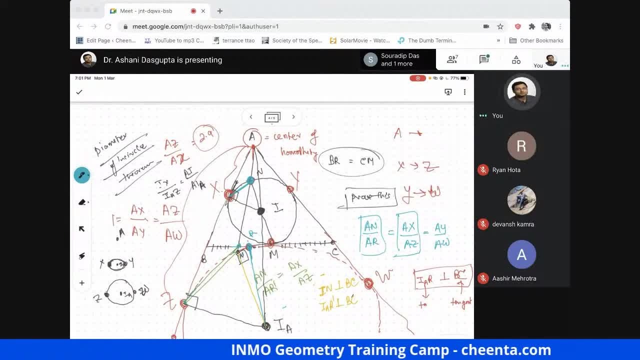 and I are prime would be the same straight line. I a are and I a are prime would be the same line segment. still is the contact point of the encirclement BC. yes, and odd is the contact point of the x-circle and BC. so I would say that mm, mmm is perpendicular. 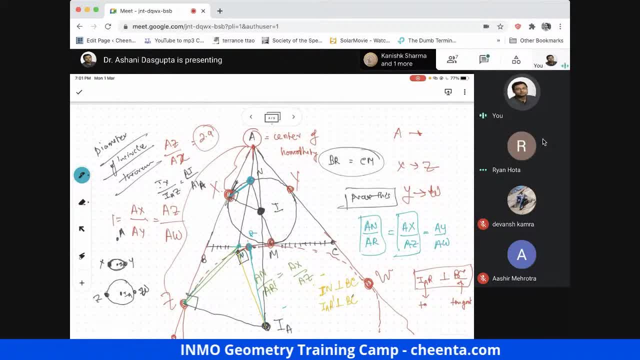 to BC. right, MM is definitely perpendicular to BC. yes, there for Ian is also a to BC, I n is for I n for knock. food is perpendicular to BC, is orthogonal to Naing arising Unearthered linearly to EC. Michael is of a diciendo belowclimbing between A, r and htc, v, LolH. might I need syста? the left lightcard tastes bad. 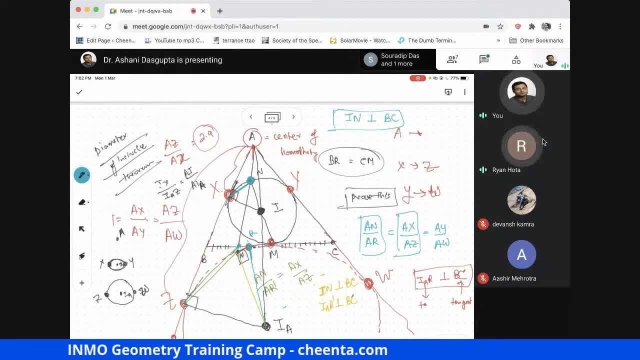 orthogonal to BC. yes, by this time you are. you are sort of familiar with lines which are not intersecting directly and think about them as perpendiculars. okay, go ahead. I a are prime is therefore perpendicular to BC. I a are prime is therefore perpendicular to BC because it is a map of I? n under the homothetic. yes, 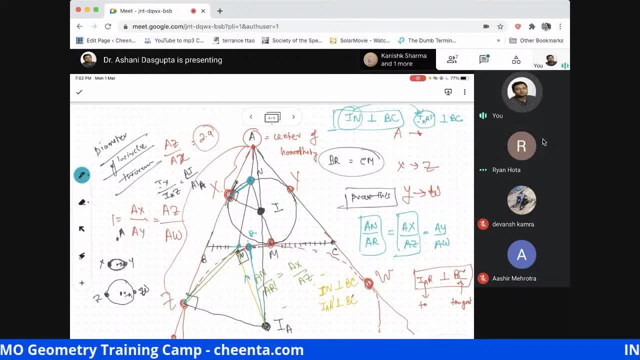 preserved. its direction is preserved because, of course, yes, with respect to BC, I a are prime and I are both. I a are, both are perpendicular. how can that be from one is BC, W, EC is parallel to ZW. we cannot say that. no, not necessarily, because Z w, az is equal to a W. if BC is parallel to ZW, then a B would be equal. 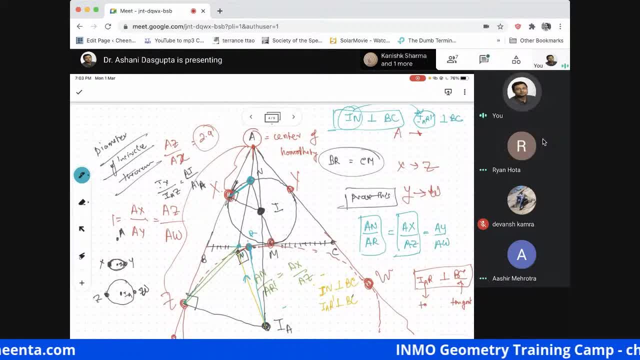 to AC, which is you only true in an isosceles triangle. so generally not okay. so i a r prime is e is equal to i a r. fantastic, so we just did the entire thing using homothety. so we now know that r and r prime are. 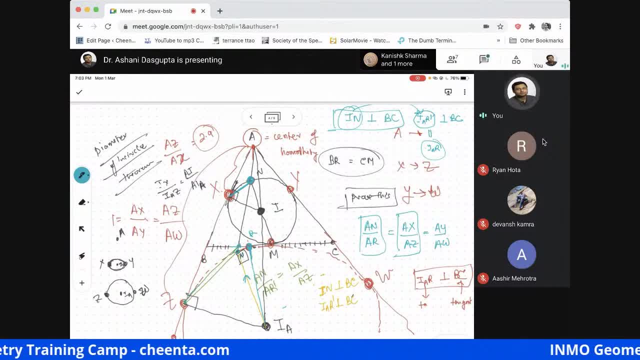 the same point, and indeed the map point n is taken to this point. r? huh, this is good, very nice. how would that show that v? r is equal to mc? v? r is equal to mc. how do you show that i'm out of time? but how do you show that? can you quickly show that? 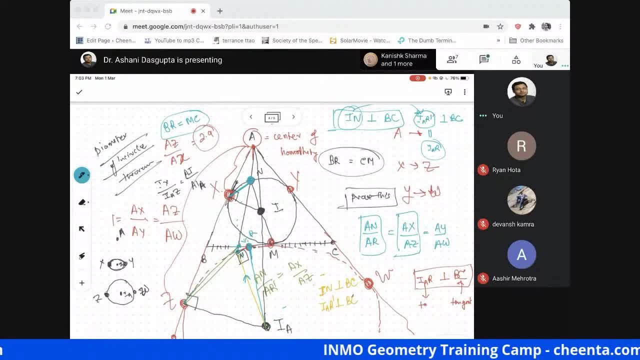 it's just one line. how do you show that? okay, so so what's? the vr is equal to mc. quickly show that vr is equal to mc. which one is v, b for bombay, vr, vr? so we, i think vr equals mc. so because there are some standard results,